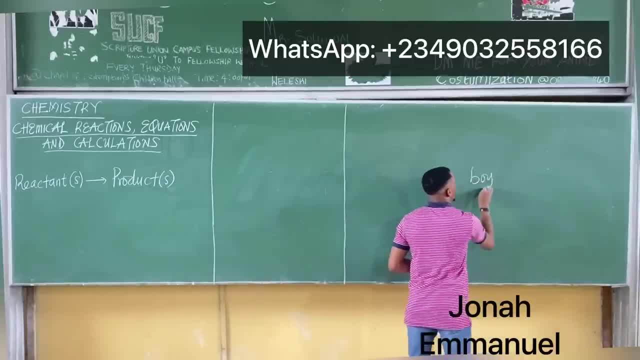 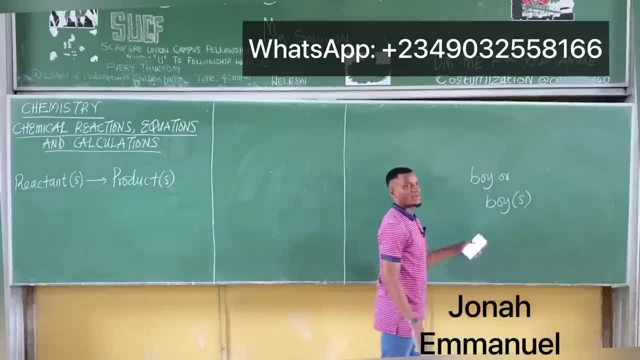 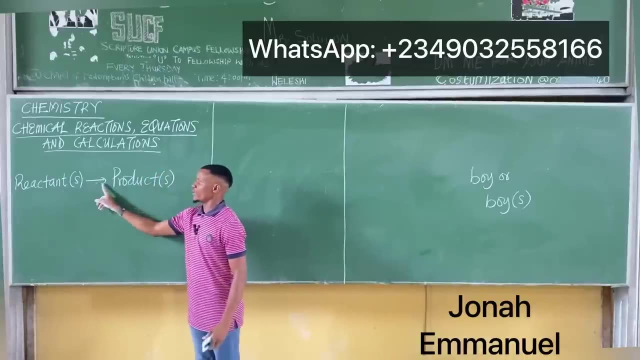 So in English language you don't write boy or boys. No, that's outdated. You simply do this B-O-Y, this: This is read: boy or boys. So this means reactant or reactants undergo chemical reaction to give you. 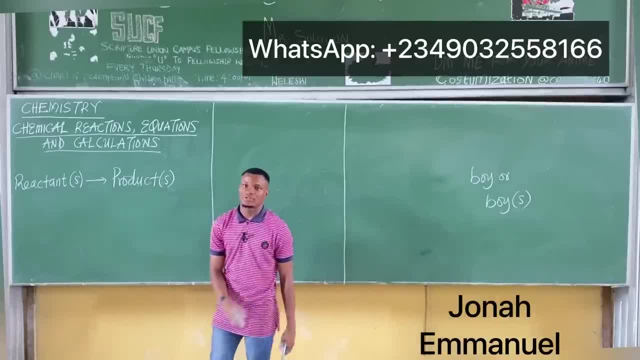 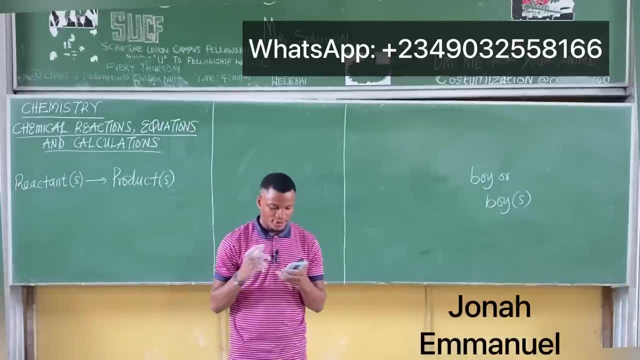 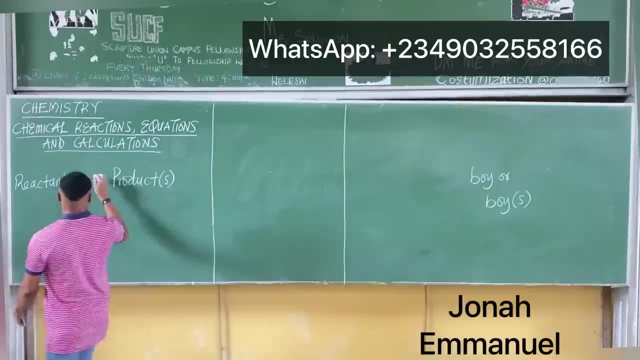 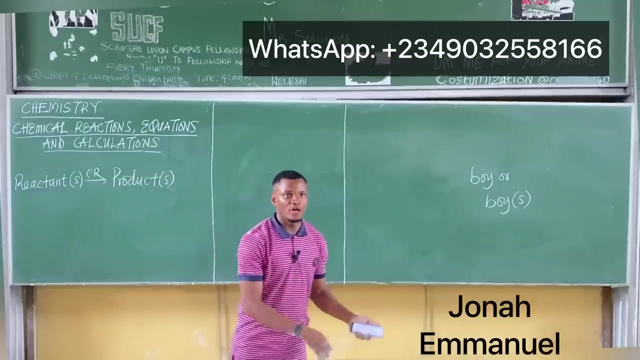 a product of perhaps several products. That's how it's written. Take down, please Take down Some visual changes. So what should be here is chemical reaction. Let me use CR Chemical reaction. Reactants undergo chemical reactions to form either a product. 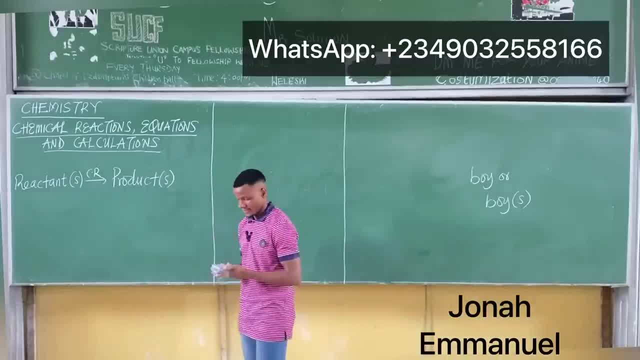 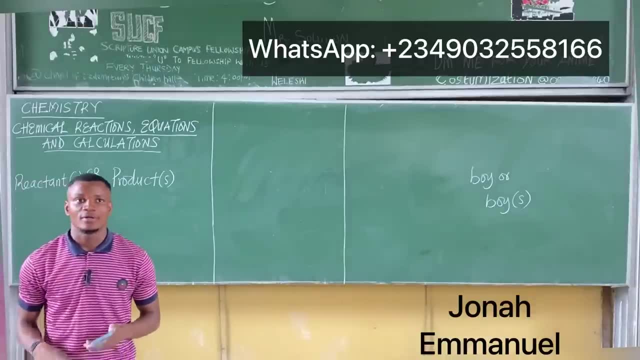 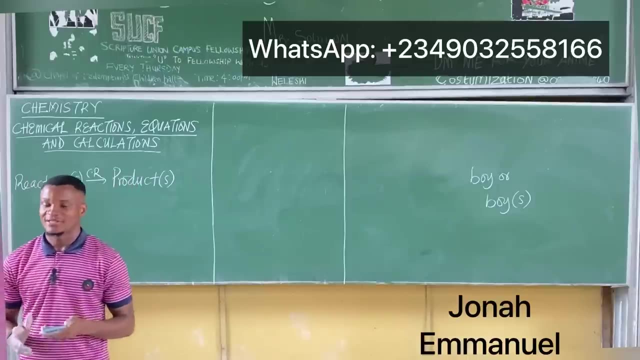 or several products, as the case may be. please Take down, please, Some visual changes that may occur during a chemical reaction includes another very important concept you should remember. Some visual changes that may occur during a chemical change or a chemical reaction includes number one. 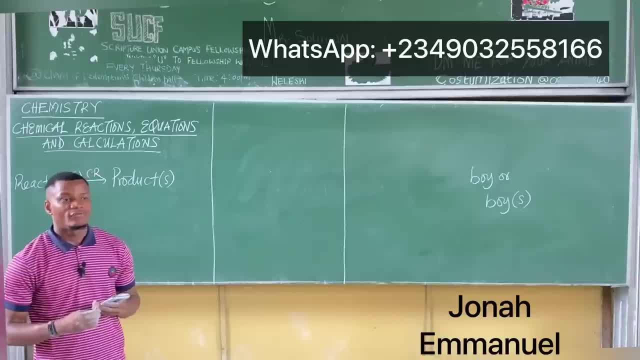 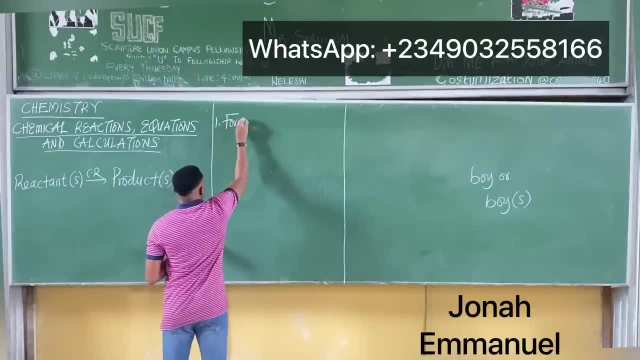 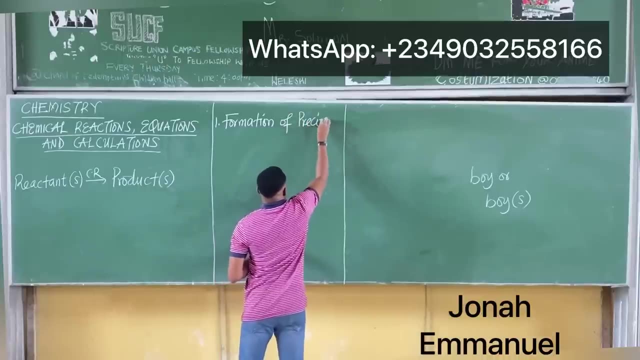 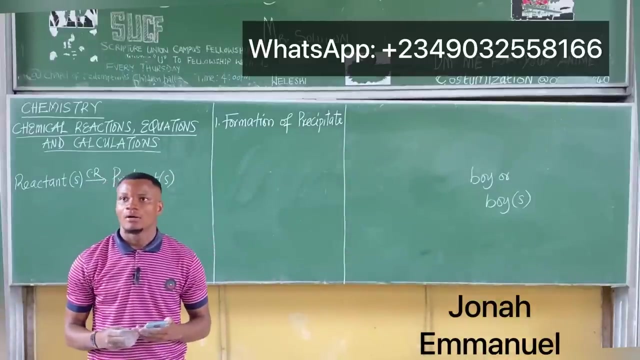 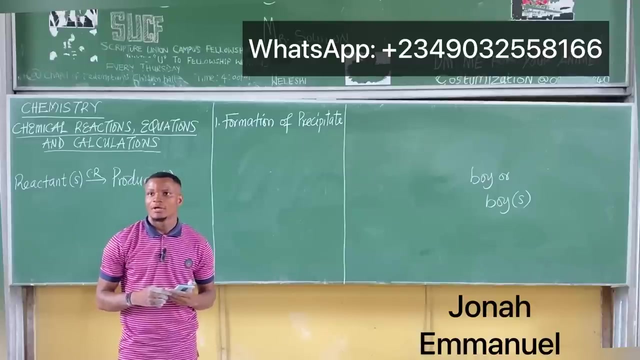 number one: formation of a precipitate. Number one: formation of a precipitate. What's a precipitate? What's a precipitate? A precipitate is simply an insoluble solid in a liquid. That's it. A precipitate is a precipitate. Short form. 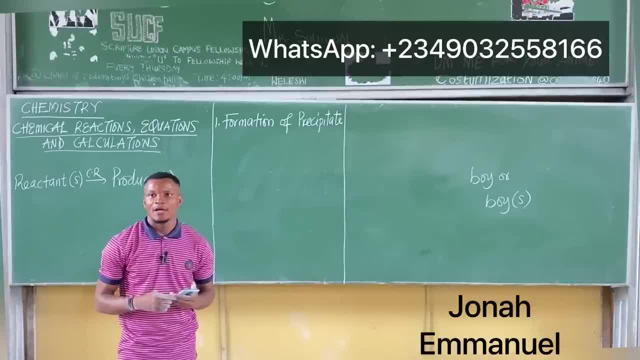 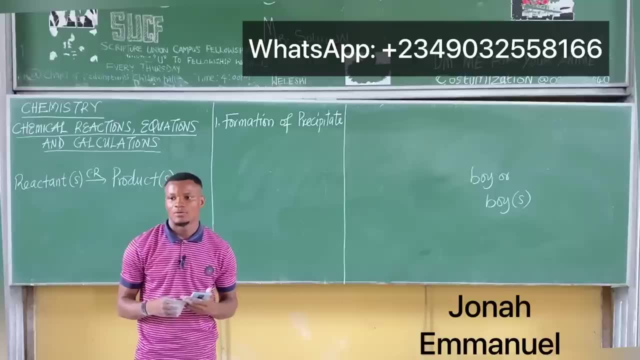 PPT. Short form for it is PPT. A precipitate is simply an insoluble solid in a liquid. Somehow, Somehow That's like a basic definition: Insoluble solid in a liquid. I'm guessing you've done practicals where you saw precipitate right. 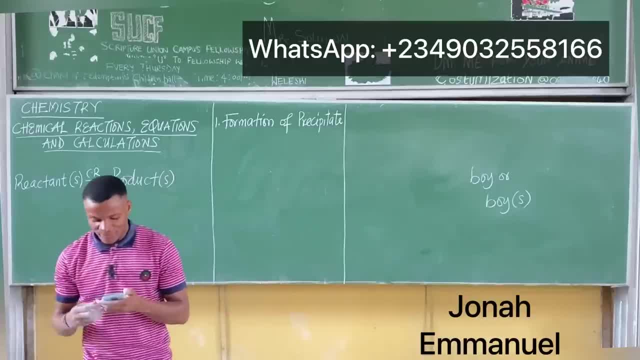 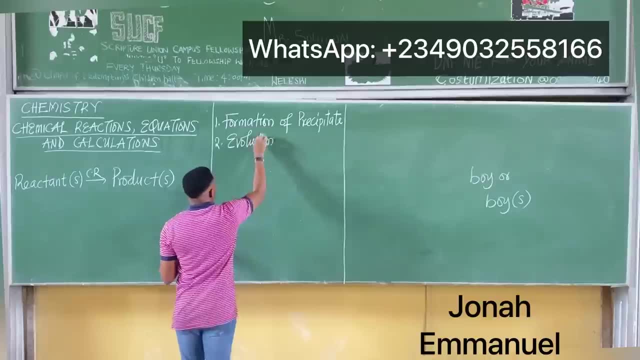 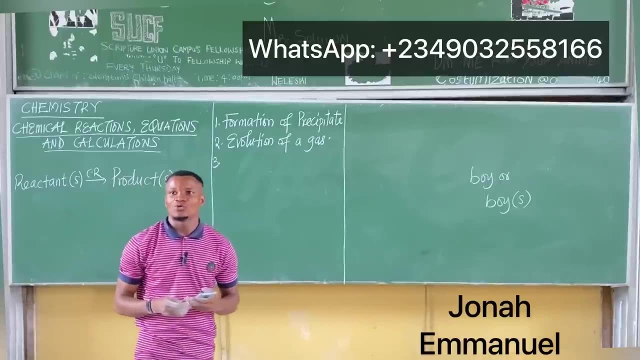 Sometimes it looks like kata, isn't it? Number two? number two: evolution of a gas. Yes, By the way, I don't know if I've told you your chemistry test is subjective and objective. It's not theory, It's subjective and objective. 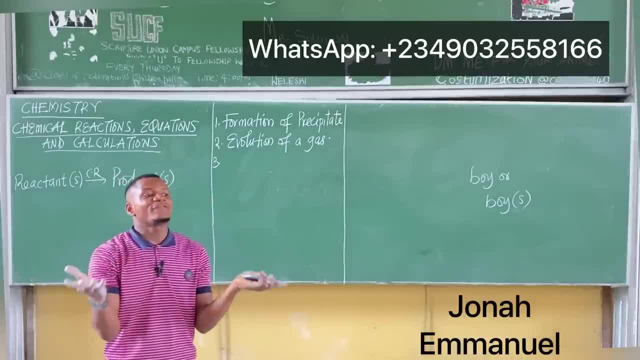 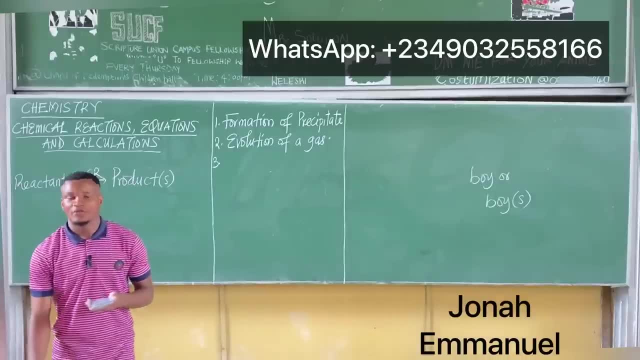 So, yeah, they'll give you the same. Which of the following is not an evidence that a chemical reaction has occurred, They'll list. So you should know how to pick this, Alright. number two: evolution of a gas. Number three: 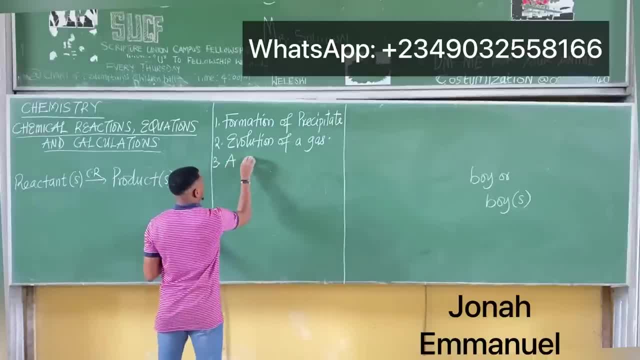 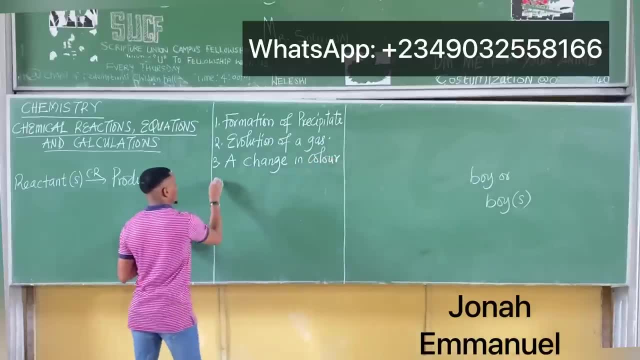 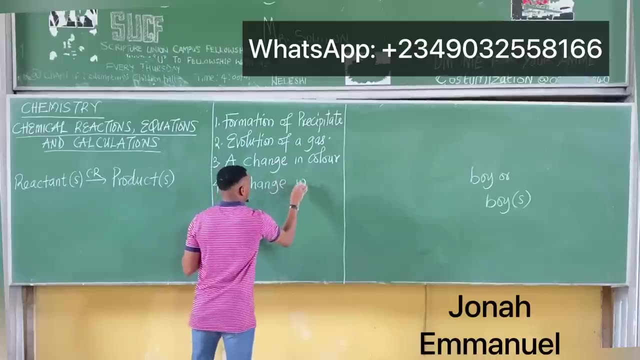 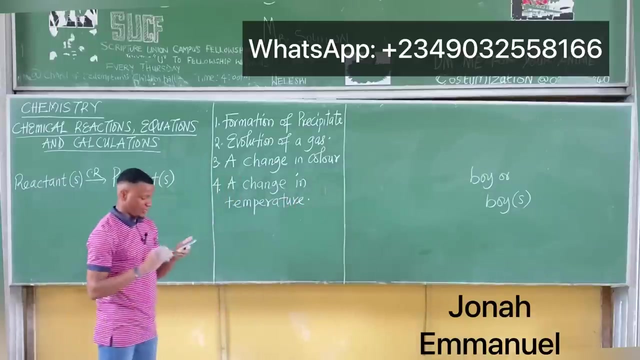 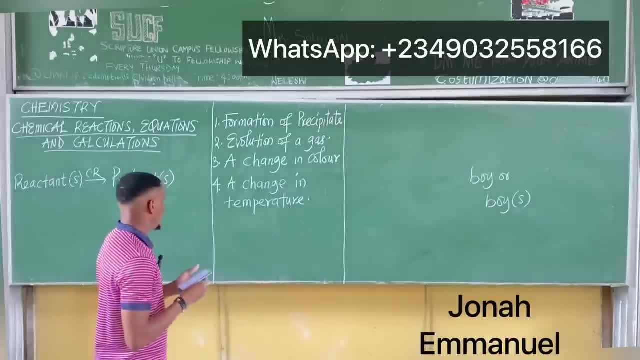 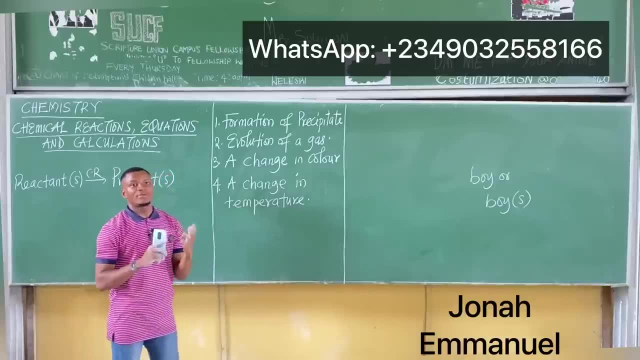 A gas is not a gas. A gas is not a gas. A chemical reaction has occurred, A change in temperature, Right. So when you do this experiment and you see PPT, that means a chemical reaction has taken place. Number two is: 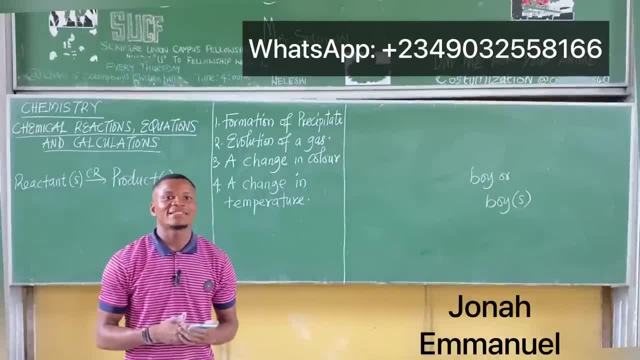 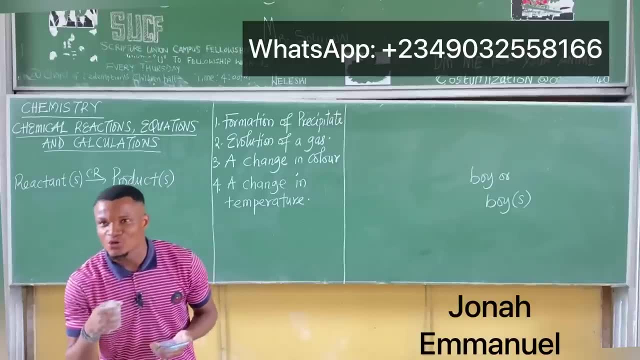 evolution of gas. When you're in the lab, when a gas is evolved, how do you perceive the gas? You don't put your nose, do you? What do you do there? You blow the air to it, is it not? 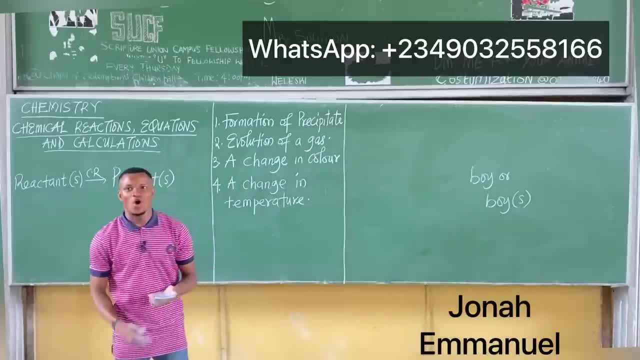 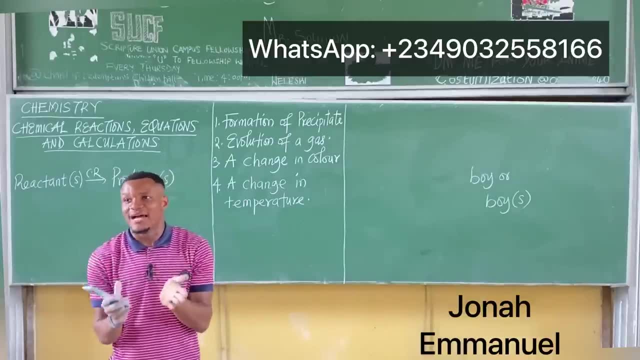 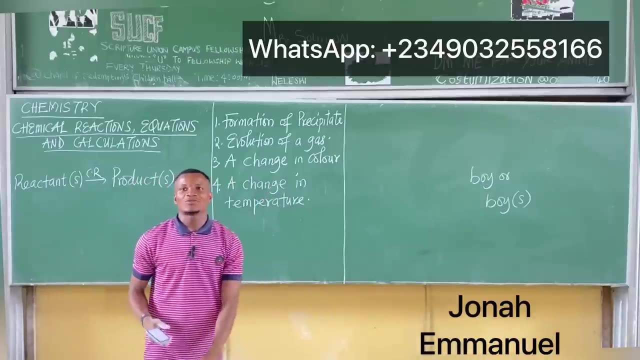 Right. Number three, a change in color. Sometimes- that's the way you do your titration right- It changes from, perhaps, orange to red. It proves that a chemical reaction has occurred. Finally, change in temperature, And that's why, in some reaction, 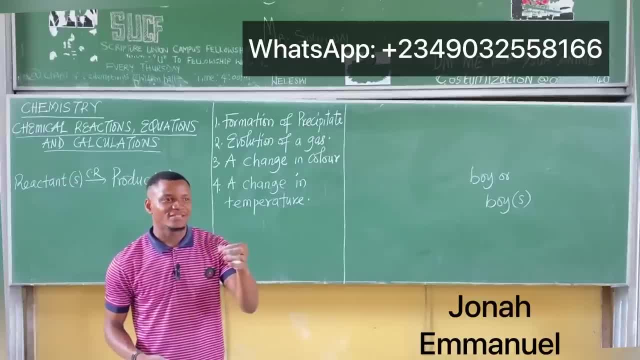 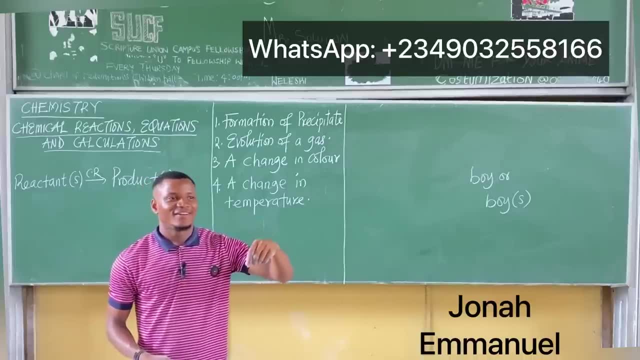 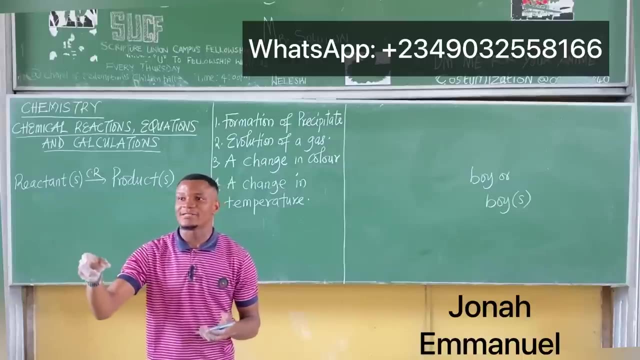 you don't use your hand to hold the conical flux. There's something you use. what's that thing called Tongue? So you use it to hold your conical flux because in some reactions, in some cases, in some cases you can have a cold substance and a cold substance. 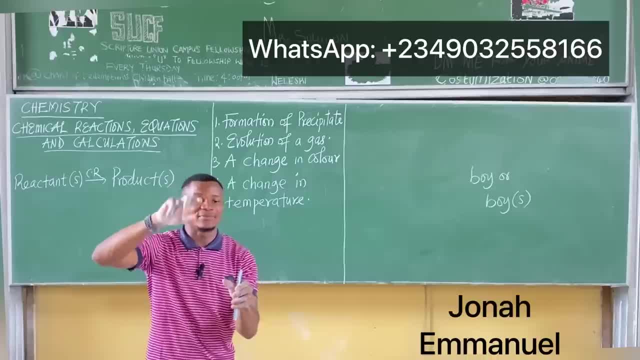 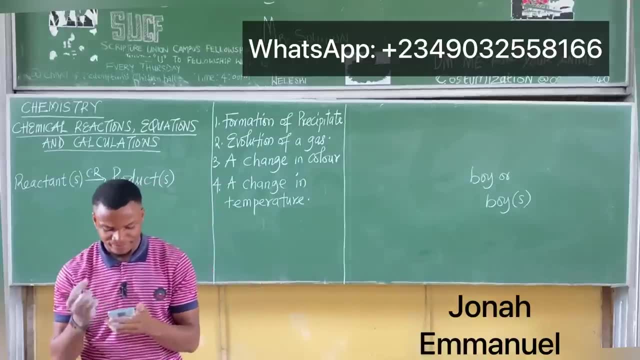 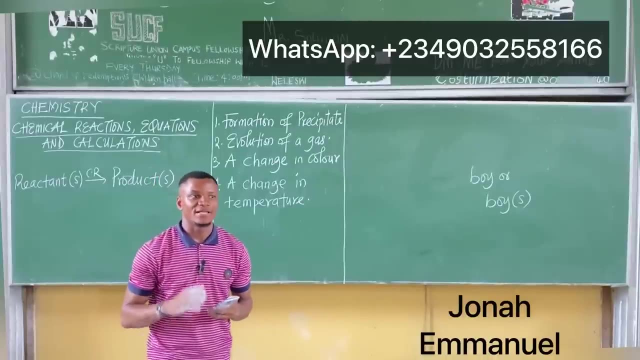 if you use your hand to hold them and put them together. sometimes the temperature can become so hot that it will fall off from your hand. you just have to leave it so you don't really use your hands in doing that stuff there. alright, step down, please, step down, please. another important concept is types of 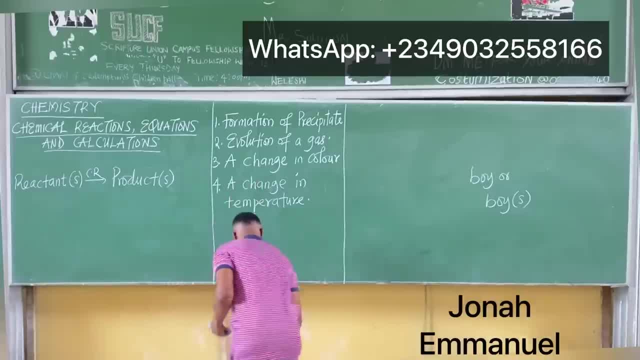 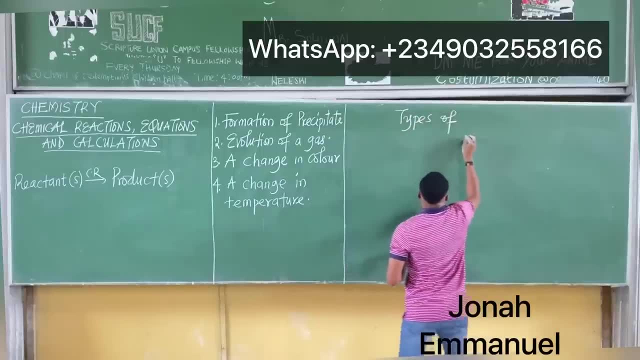 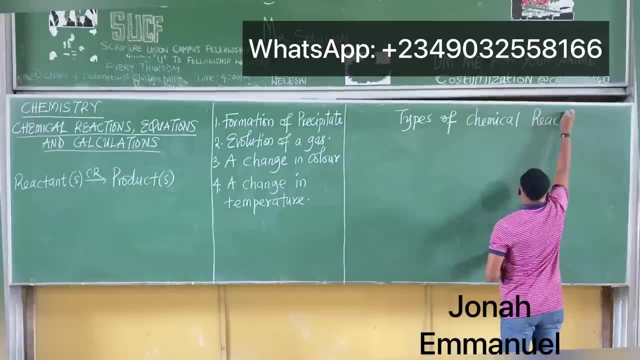 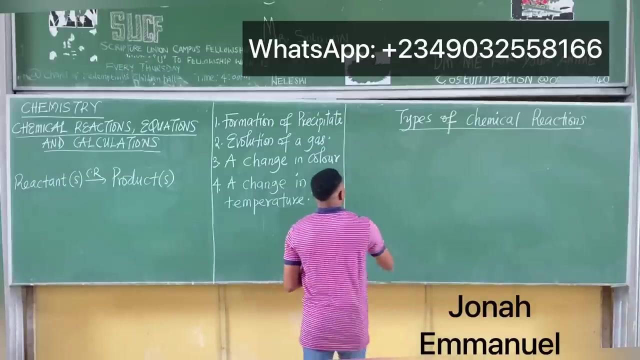 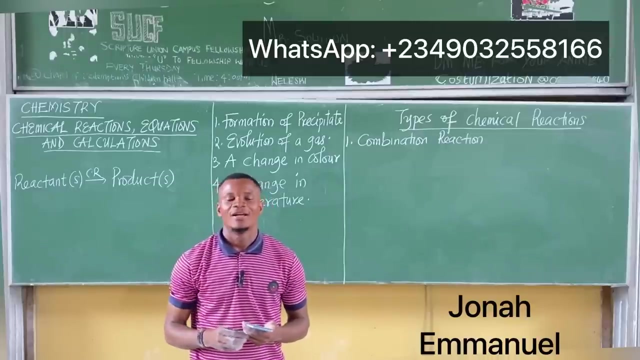 chemical reactions. please, very important points: chemical reactions. the different types of chemical reactions include number one: combination reaction. it's almost impossible to write physics exam or test now. you don't see this particular one, either your test or exam. it's almost impossible. chemistry- it's almost impossible to write chemistry. 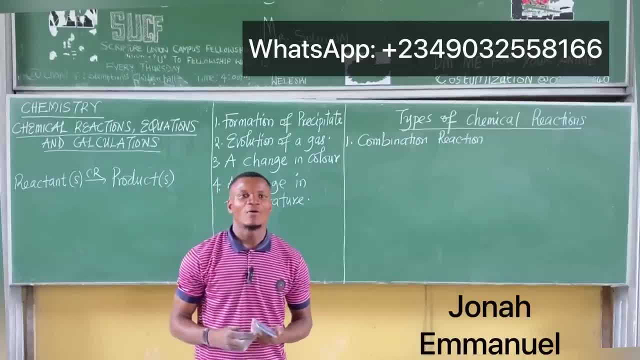 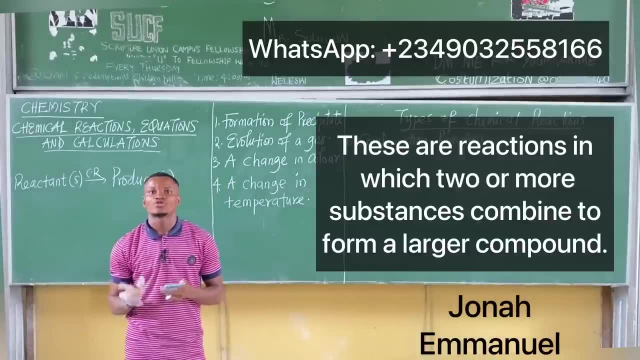 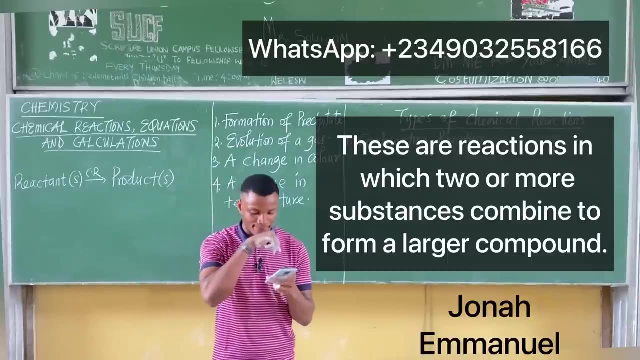 test or exam. now you don't see this concept. number 1 is called combination reaction. take that please. very short notes: these are reactions in which two or more substances. these are reactions in which two or more substances combine to form a compound. two or more substances combine to form. 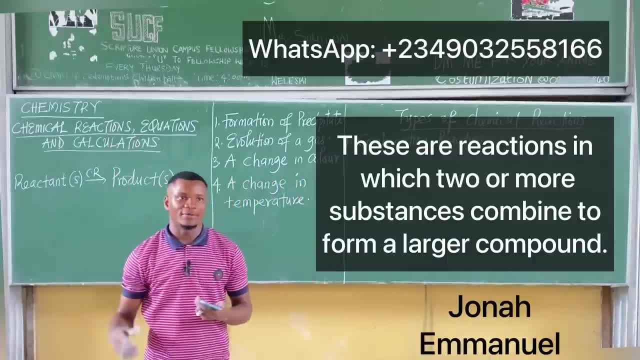 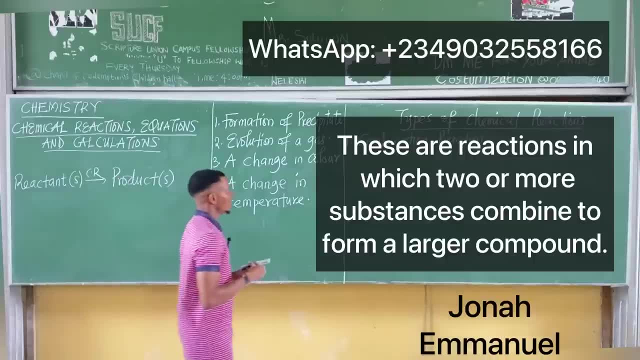 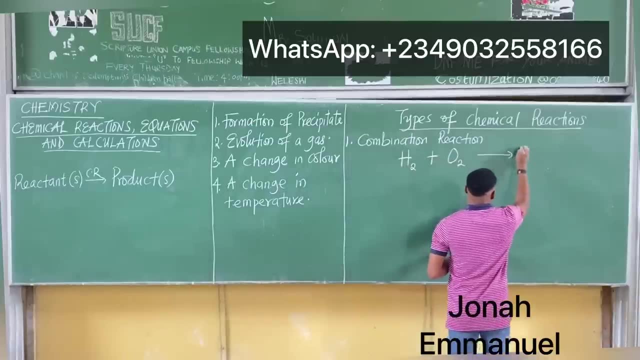 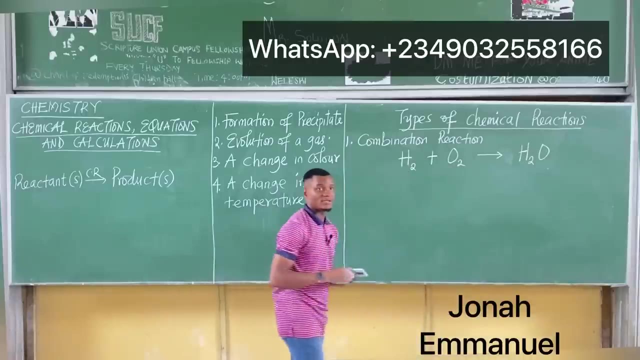 what is the word? a larger compound? yeah, better, two or more substances combine to form a larger compound, example in the formation of water. all right, so I have this, you have that. you look up, I have two balances: the water, hydrogen oxygen. I have these, I have two balances, obviously, two hydrogen here. 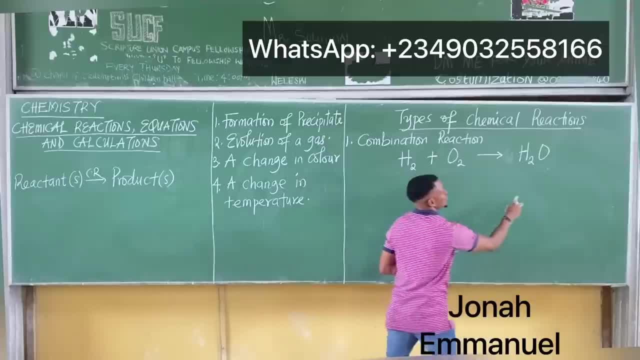 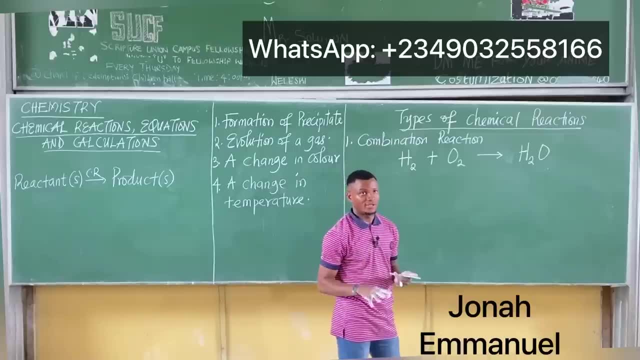 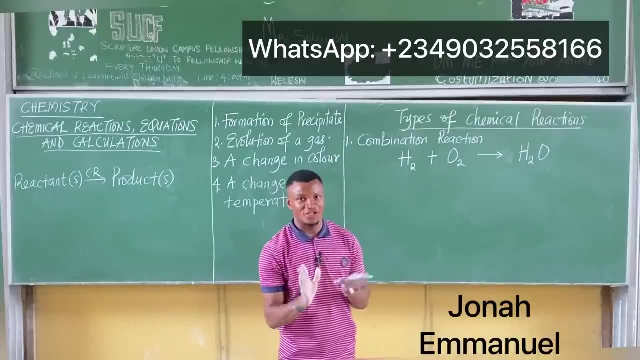 two hydrogen here and now hydrogen, but hydrogen declined here. two hydrogen here balanced. two oxygen here. just one oxygen here. please, at this level, level 100, you don't balance chemical equations by adding subscripts. you only use coefficients in quotes, whole number coefficients. listen if I want to use. 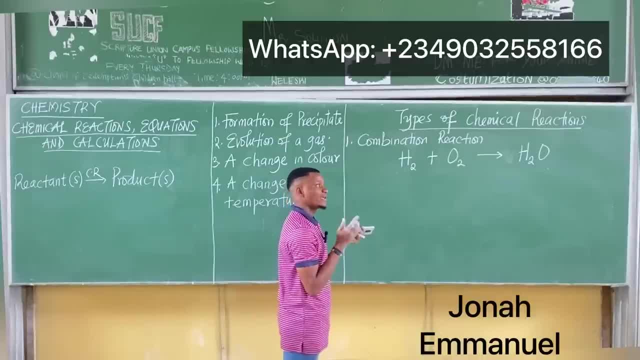 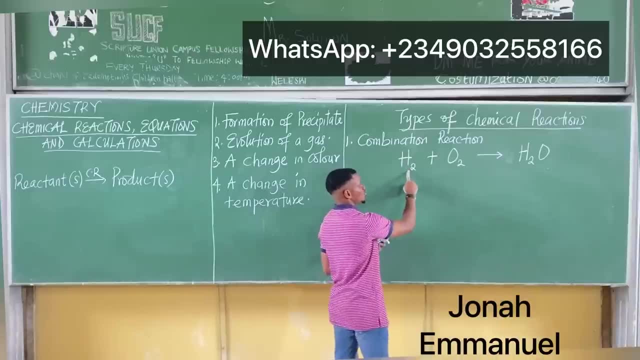 mathematics. here there are different ways I could balance this. let's say, for instance, I want to balance this one here I'm having H2. H2 balance, one oxygen. I could come here technically to say one over two and it's balanced. of course it becomes this times this half of two is one. so technically this is. 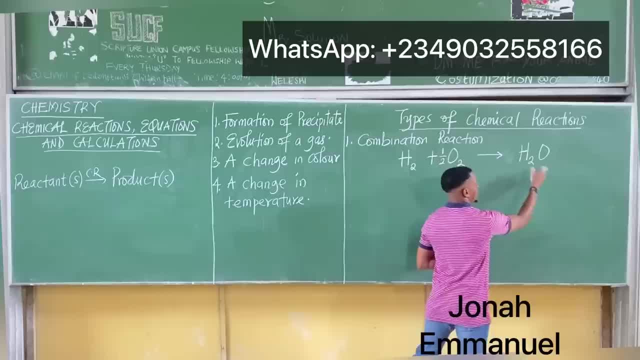 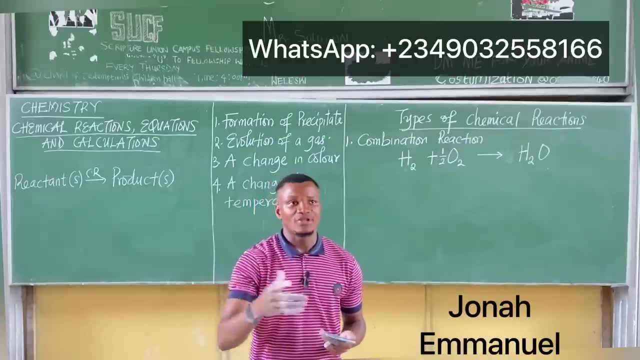 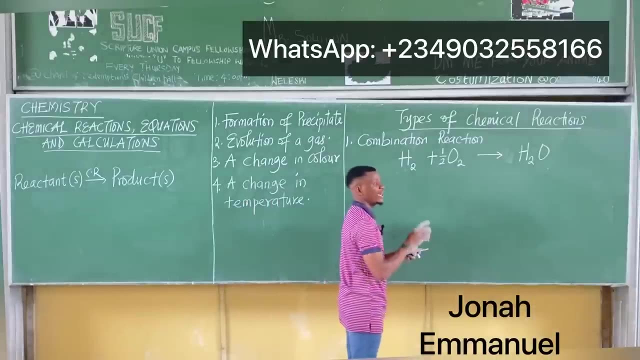 balanced half of two: one oxygen here, one, two hydrogen, two hydrogen. what is correct, please, at your level is not permitted. please, as you go higher in chemistry, it will be permitted. so, please, when it comes to balancing equation, we don't use fractions, we only use what there whole. 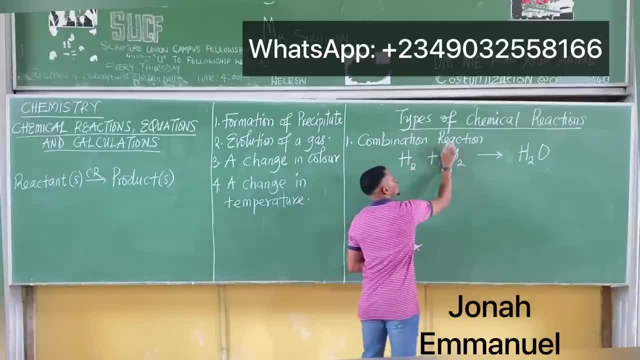 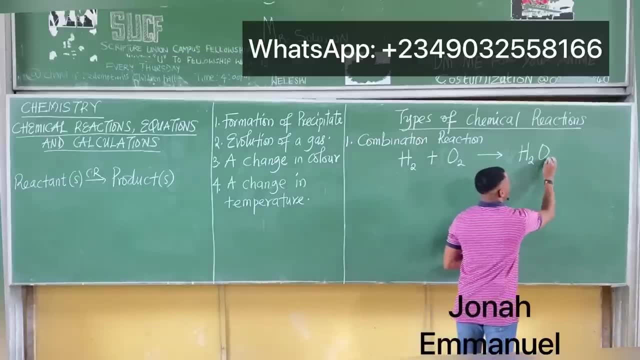 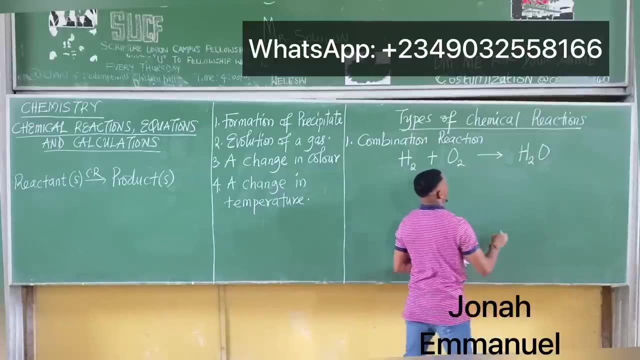 number coefficients, that's one number two. we don't use subscripts, so you don't say H2, H2, O2. you come and say two here. no, that's wrong, although this exists, yes, but this is wrong. please to balance this, of course, two, I'll bring two here. it becomes two here. 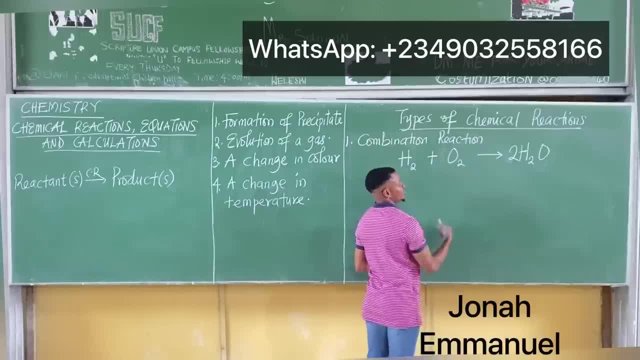 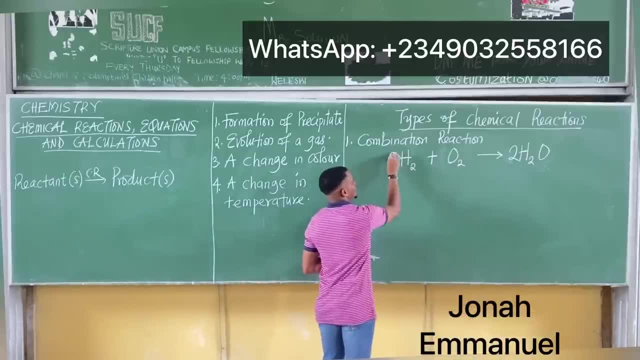 2 times 1, 2 oxygen: 2 oxygen balance, but I have distorted hydrogen becomes 2 times 2, 4 hydrogen. I have 2 here, so I'll add 2.. This becomes a balance equation for this. This is an example. 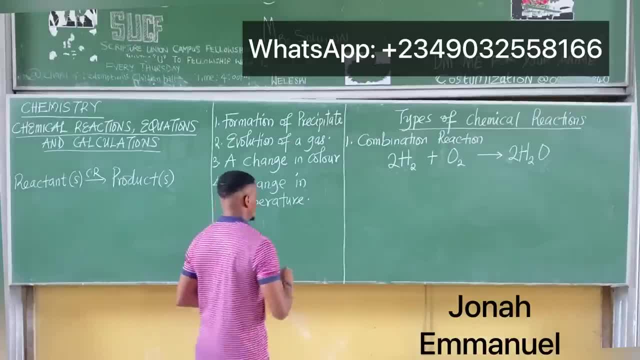 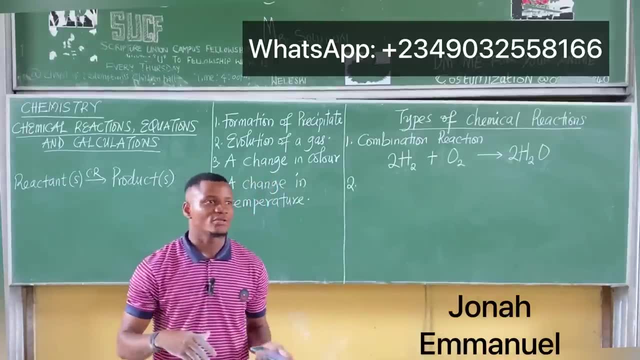 of a combination reaction. Number 2. Number 2, I'll tell you how to know if it's combination or not. So I'll give you an equation. say what kind of equation is this? How to know? Number 1 is combination reaction. 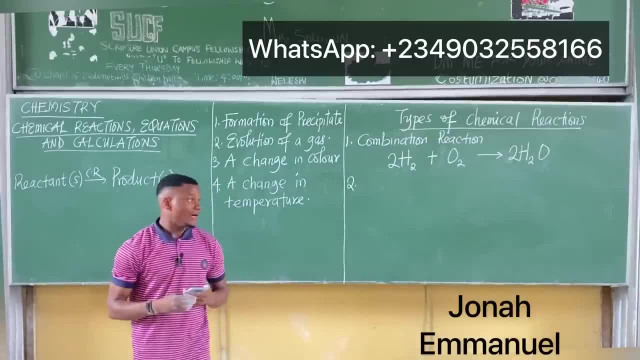 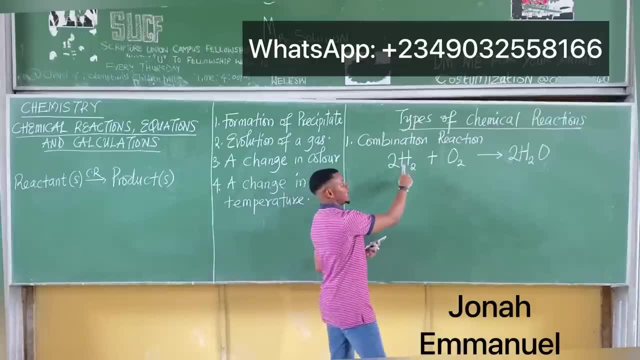 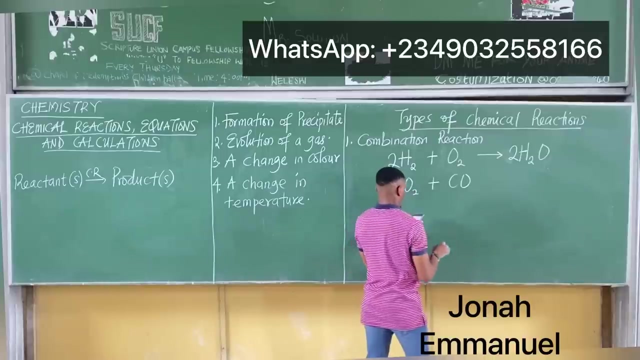 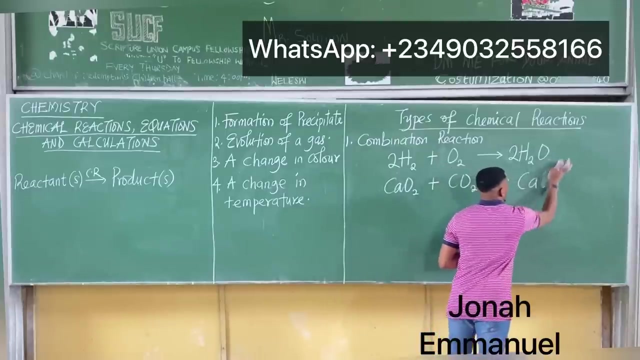 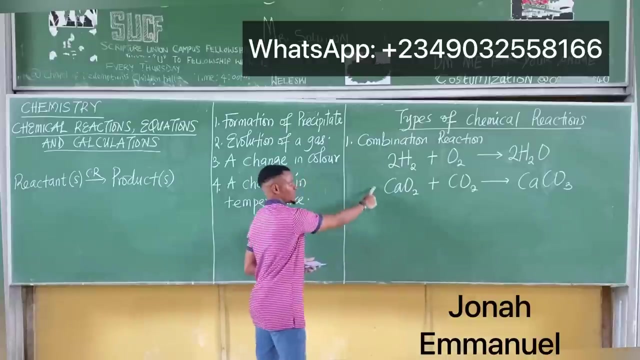 Let me state something please. For this one I have elements and elements combining to give compounds. In some cases I can have compound and compound like this, like this one here. Look at the board please. This equation here: is it correct? Yes or no? 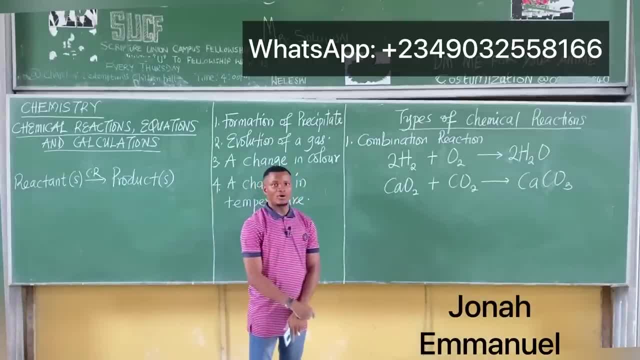 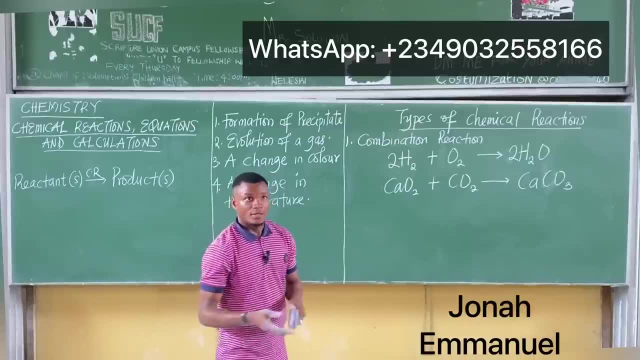 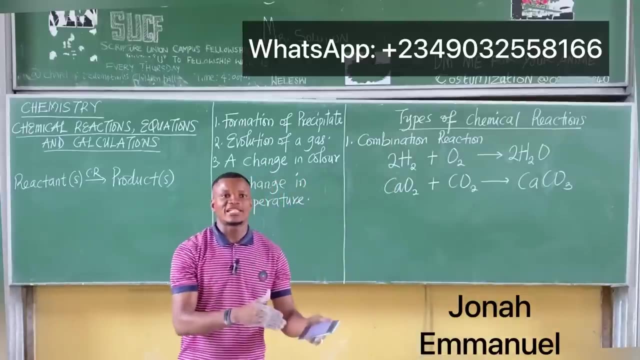 This equation here. is it correct? Yes or no? What's wrong? Okay, hold on, We have to balance. that study, That study. This equation here, This equation here, This equation here. Is it correct? No, Hold on, Is it that it's correct, but not balanced? Is that it? 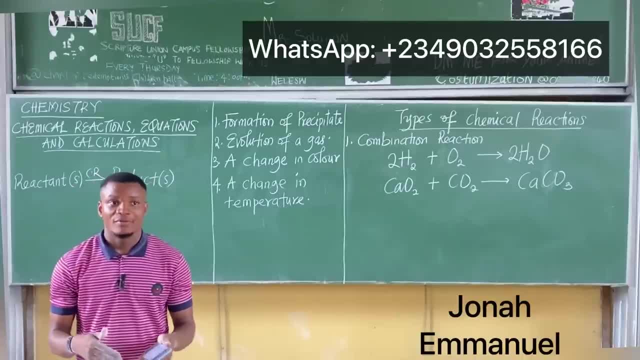 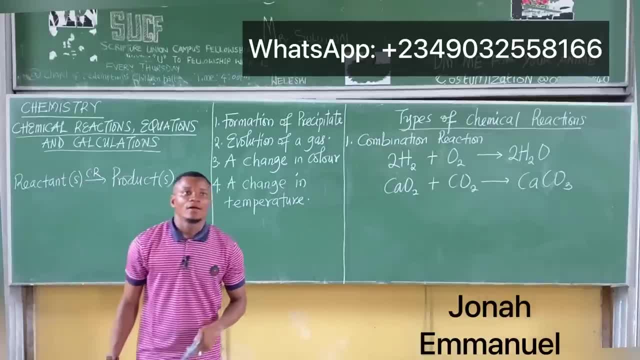 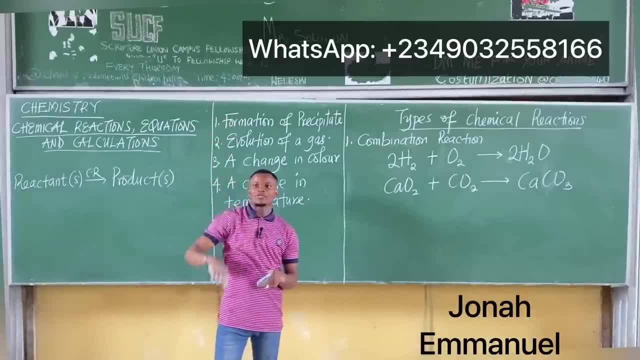 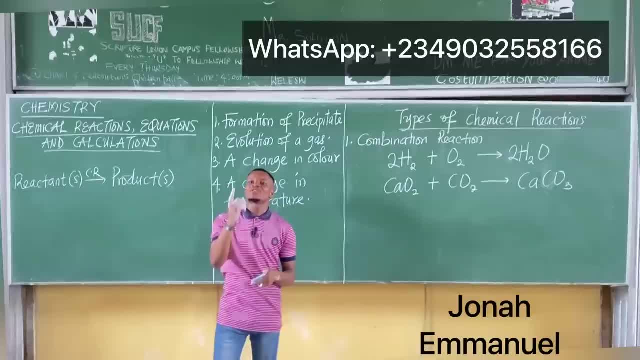 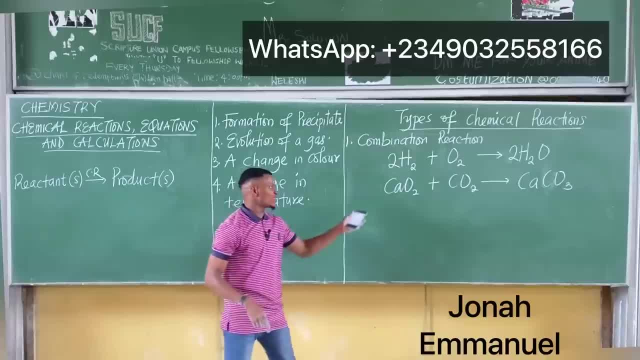 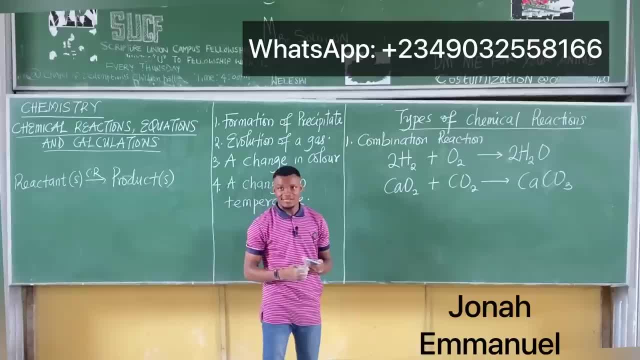 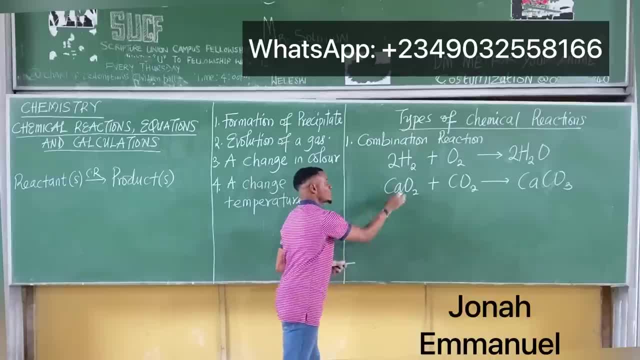 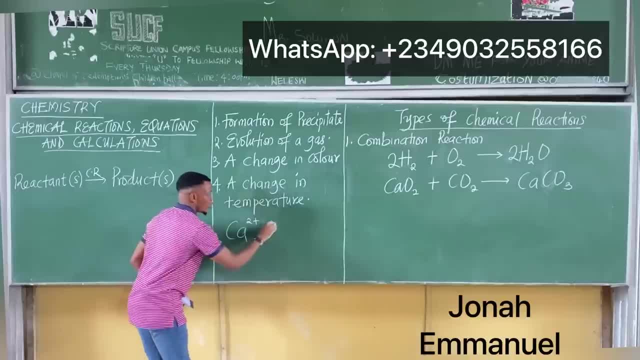 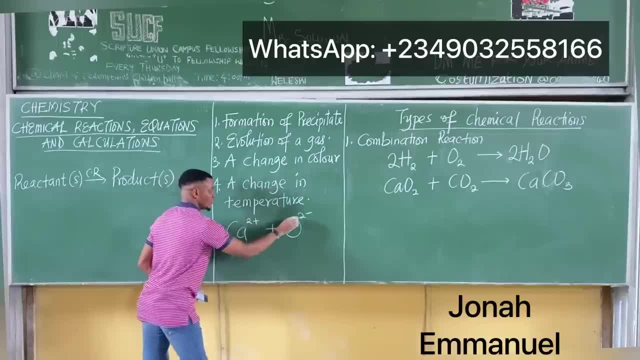 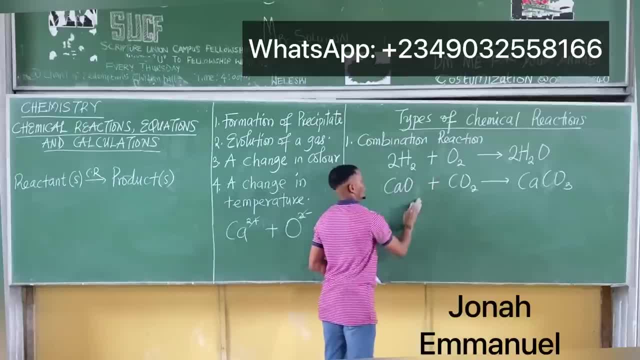 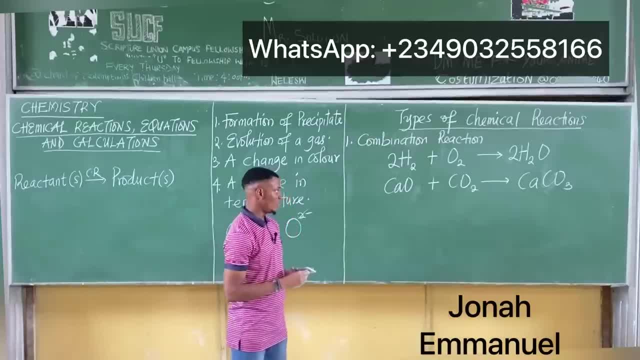 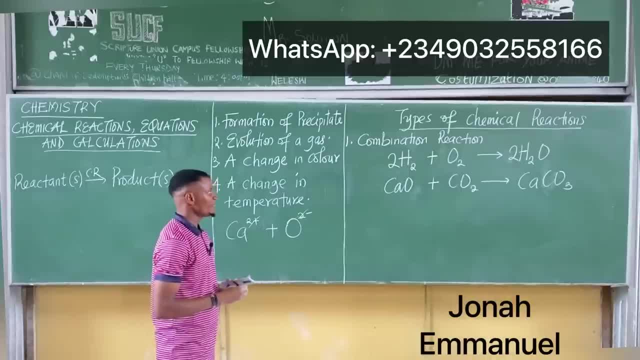 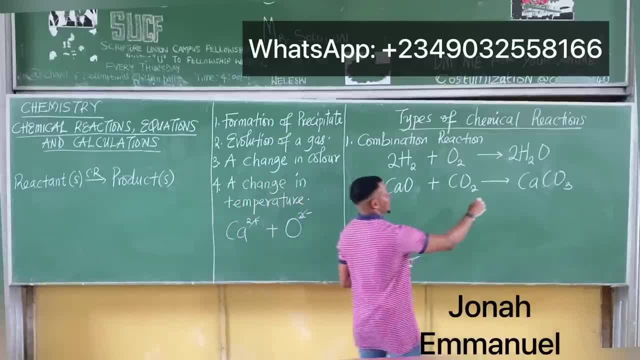 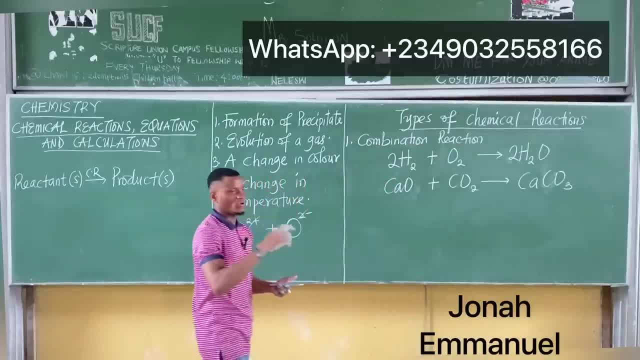 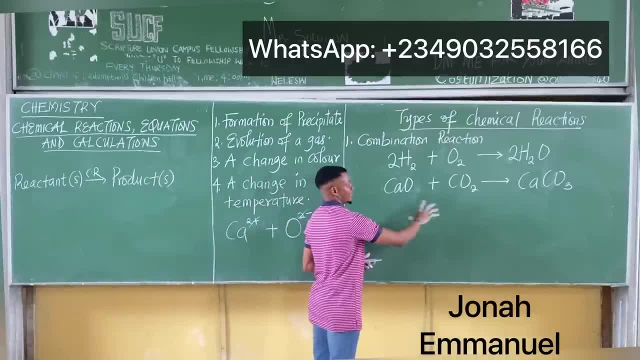 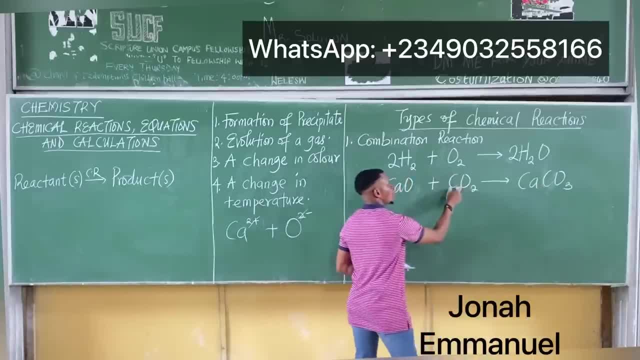 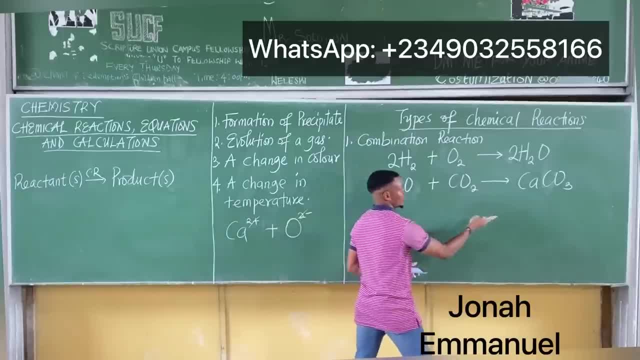 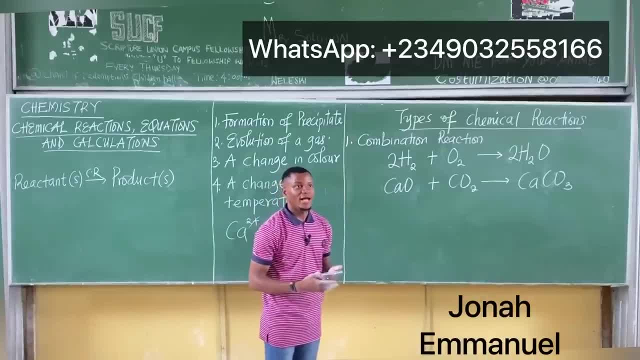 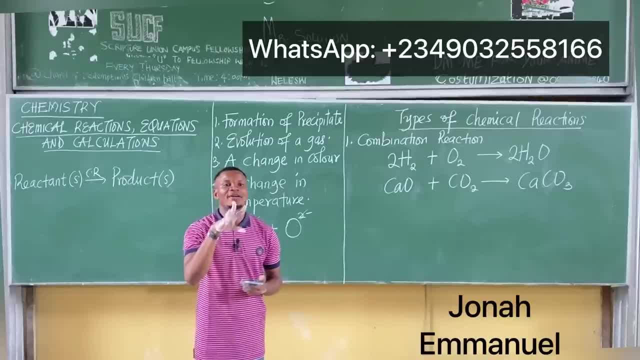 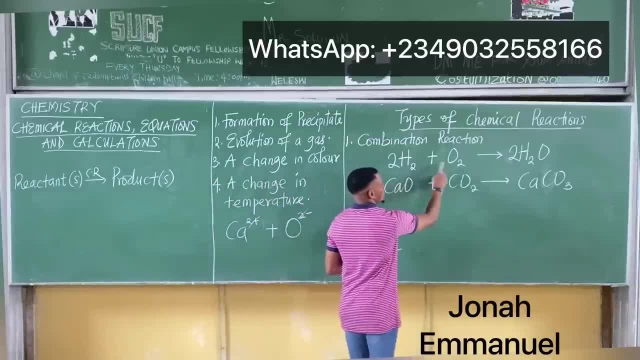 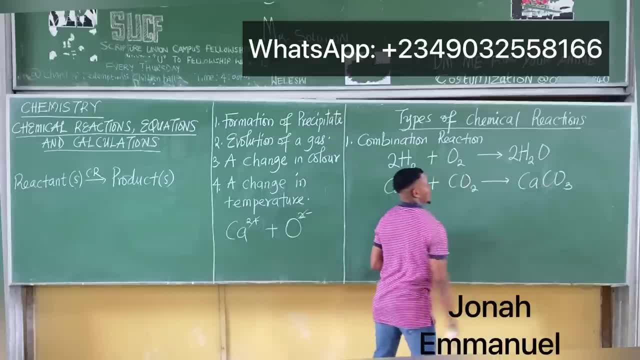 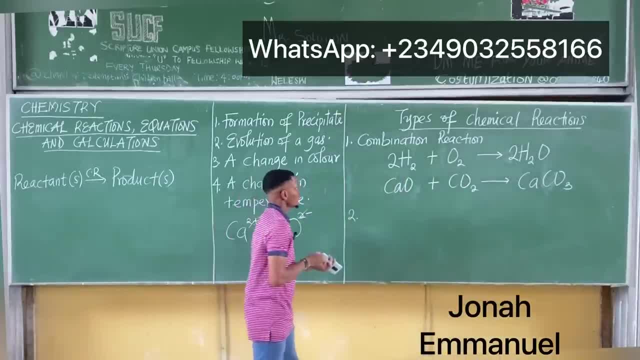 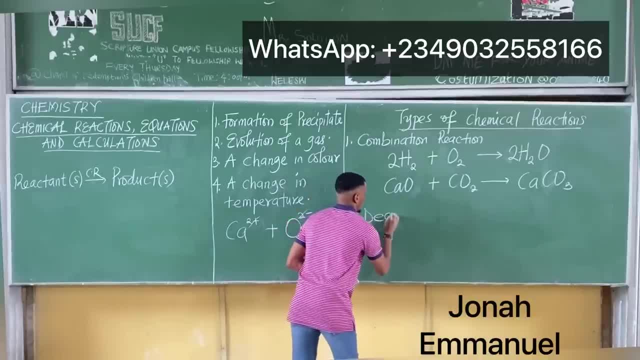 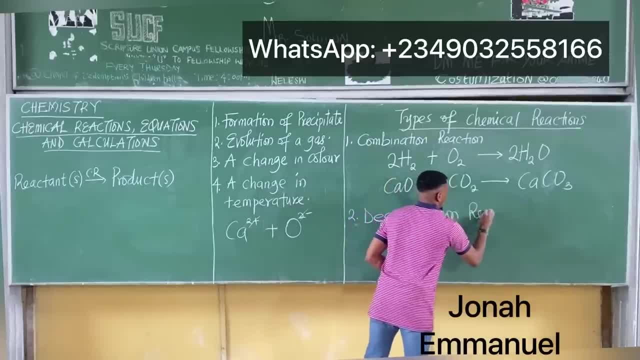 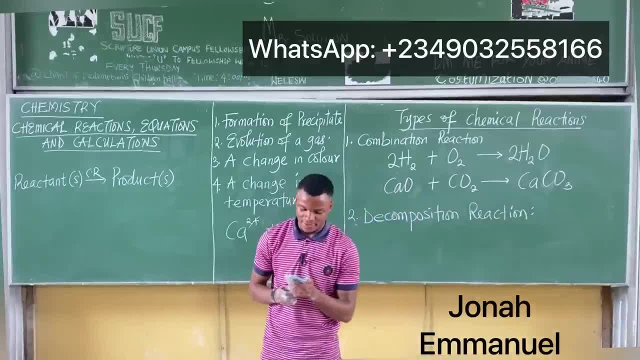 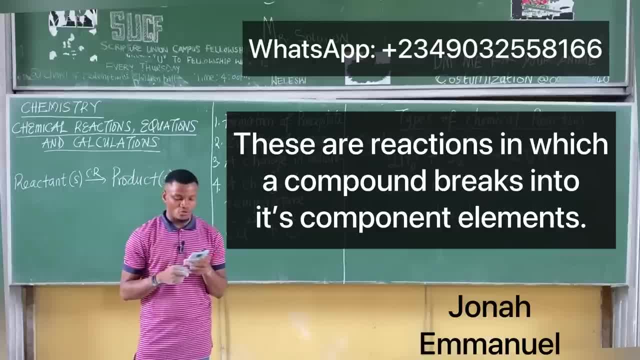 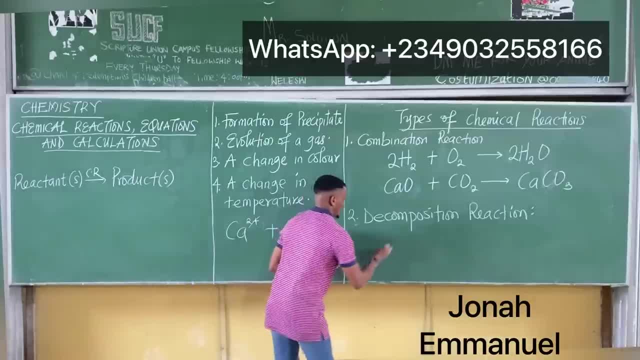 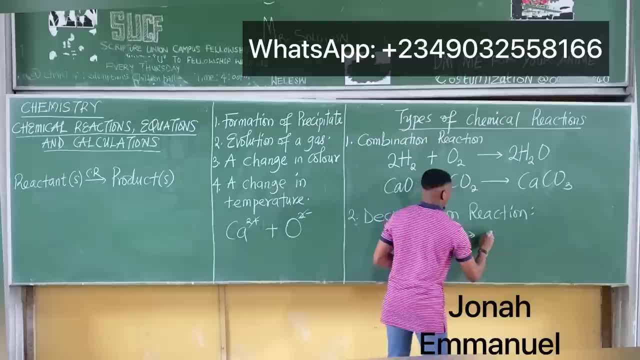 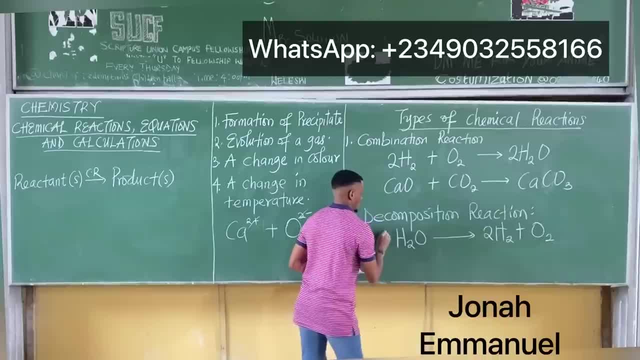 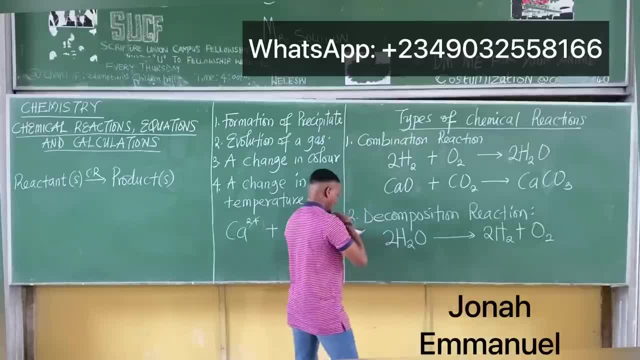 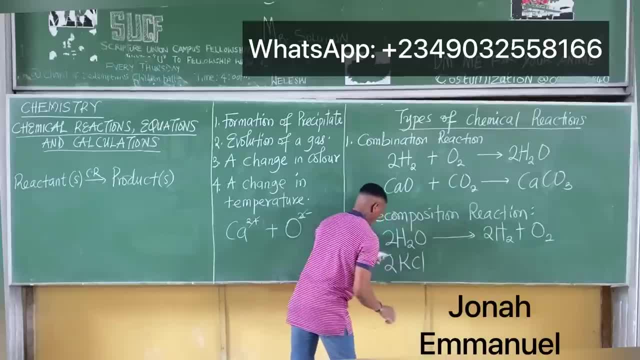 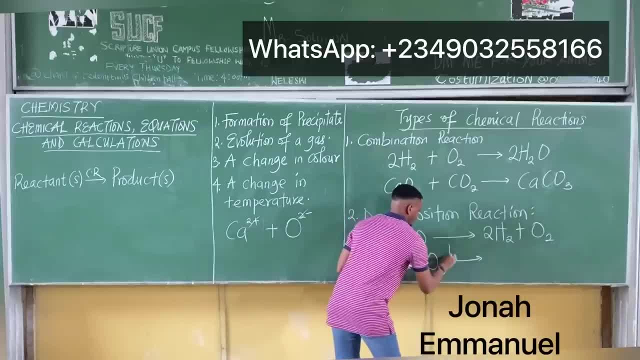 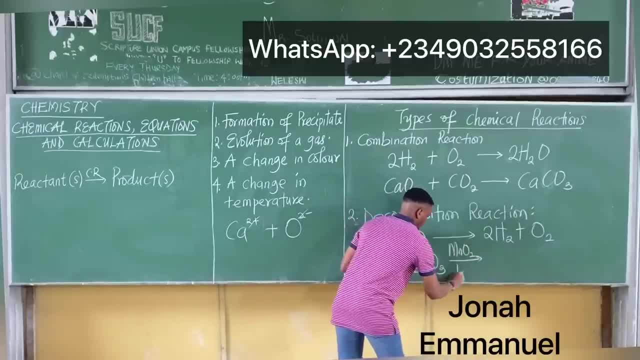 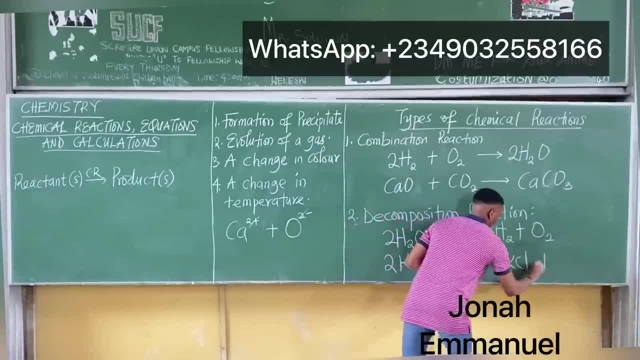 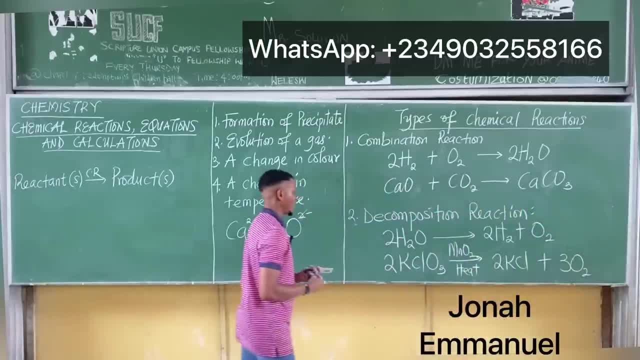 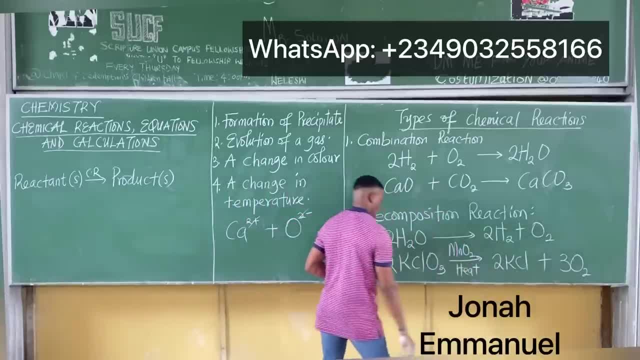 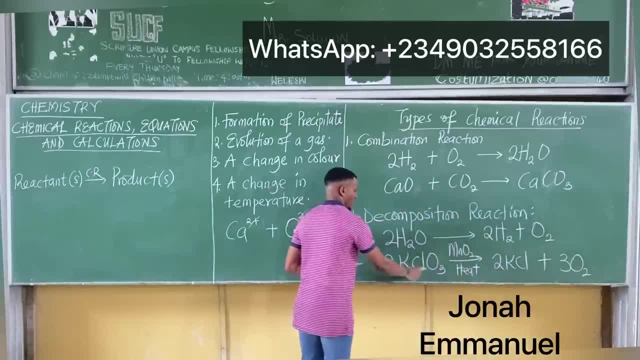 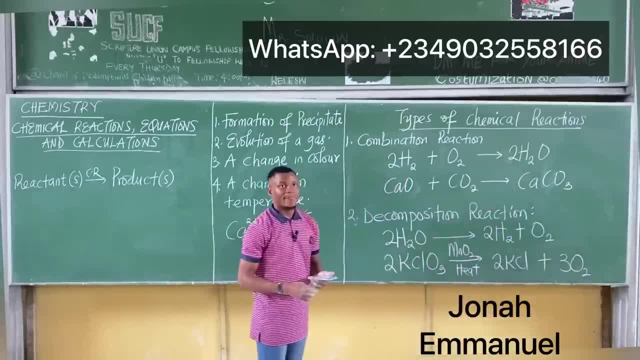 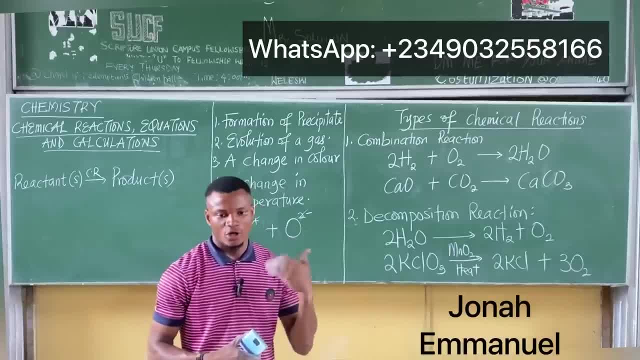 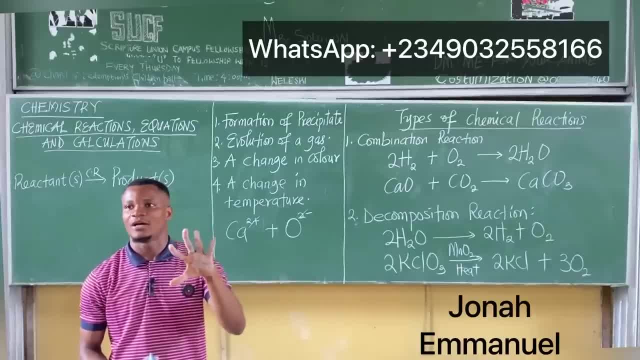 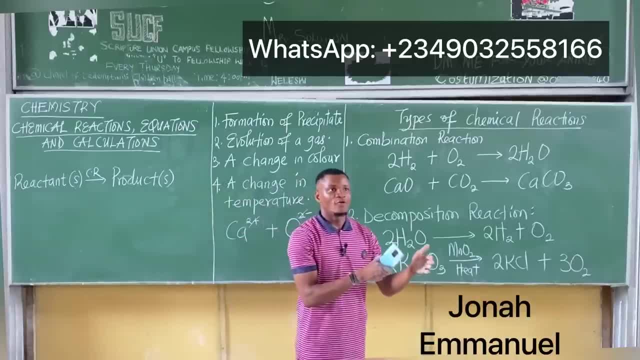 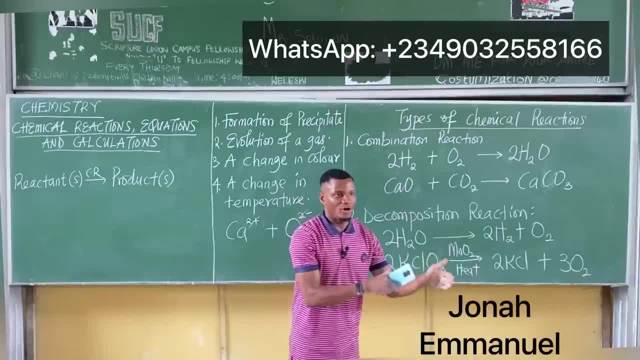 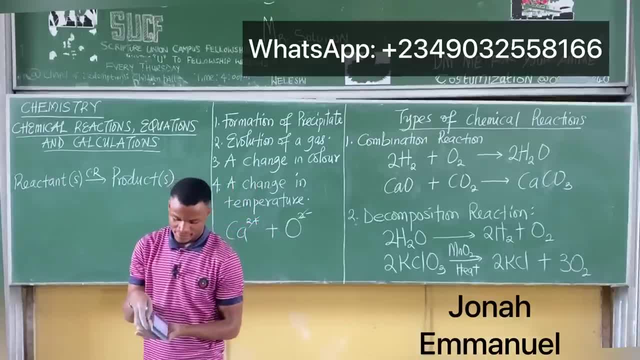 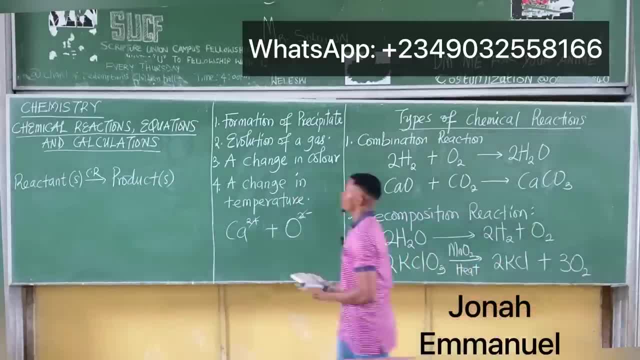 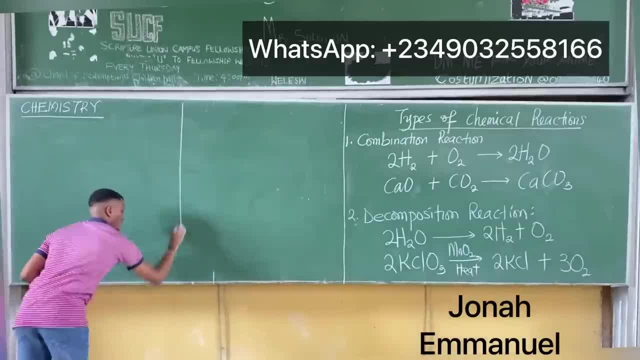 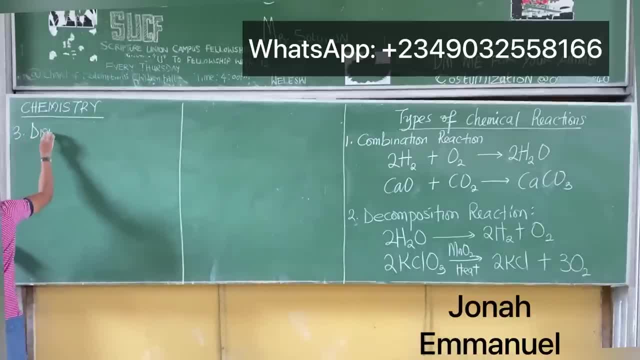 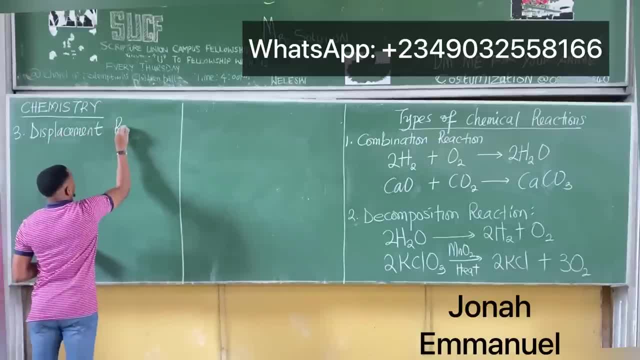 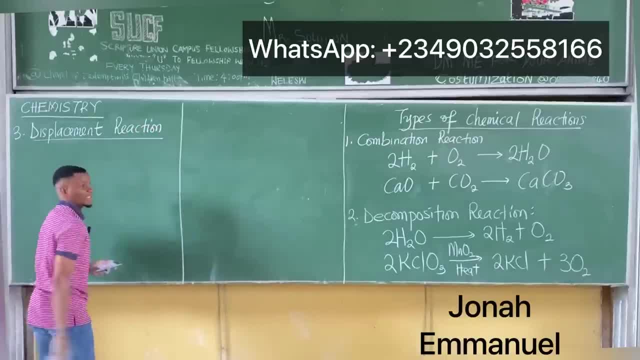 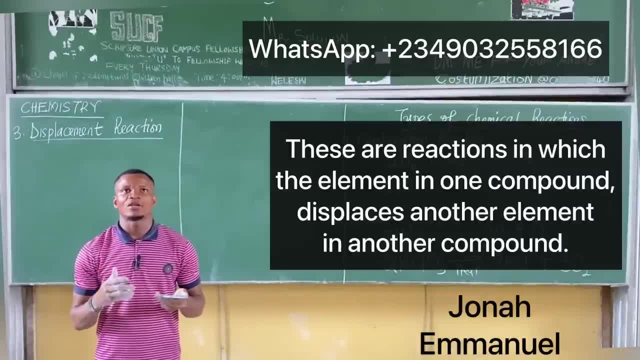 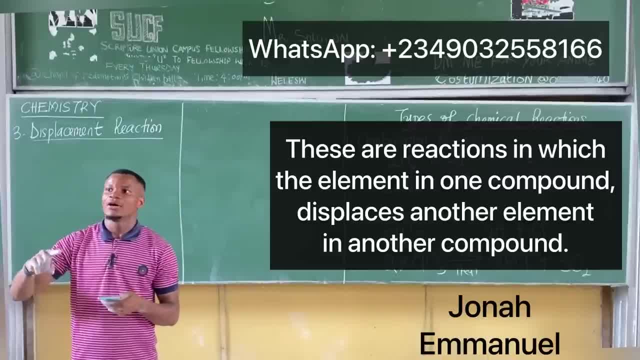 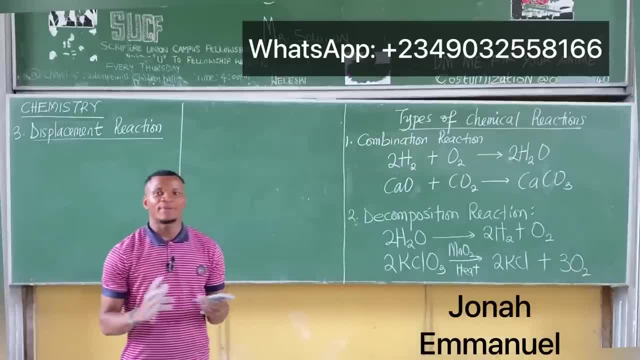 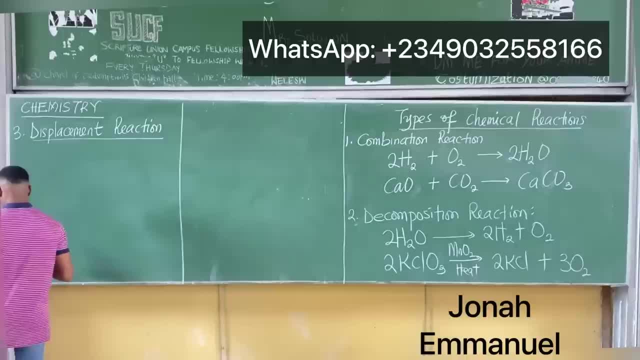 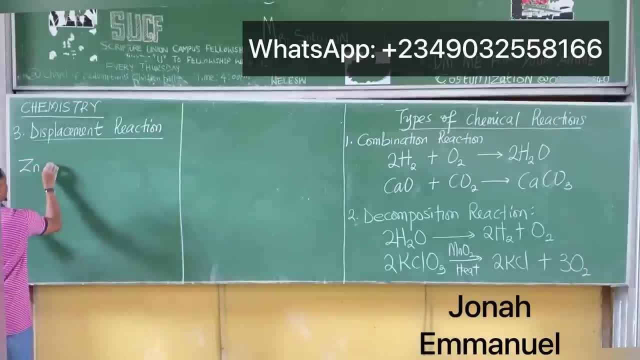 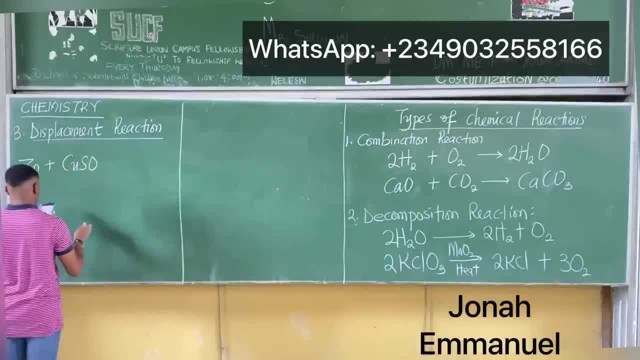 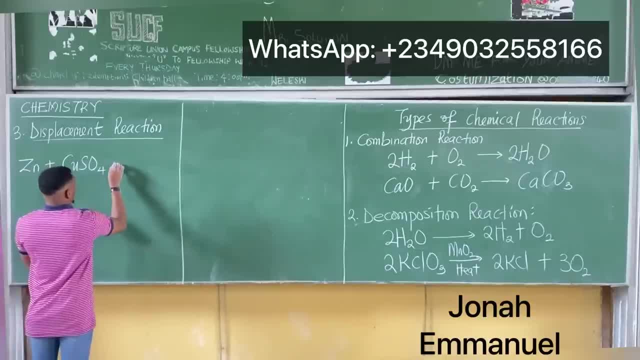 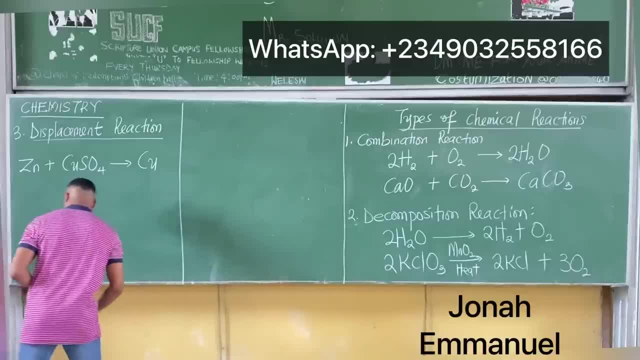 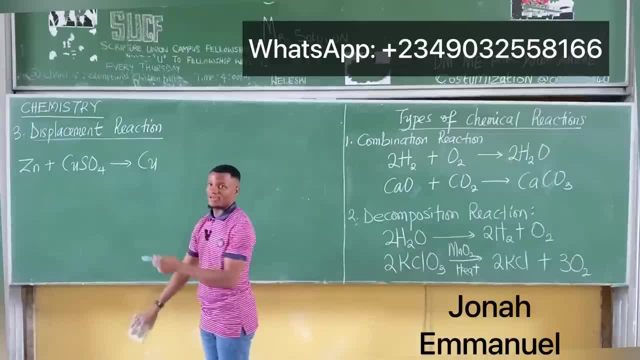 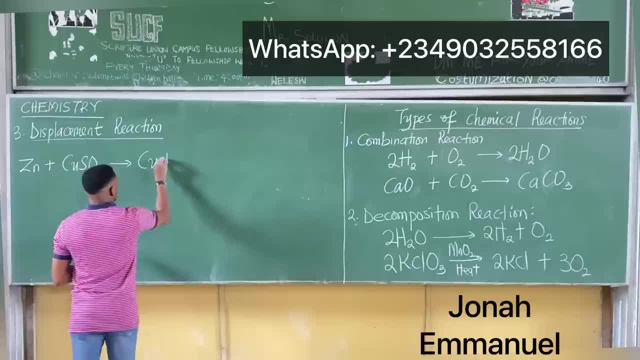 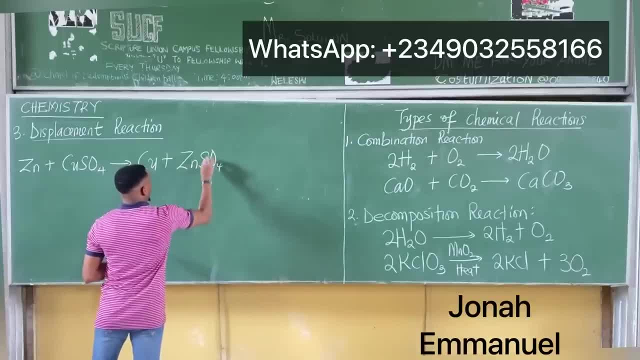 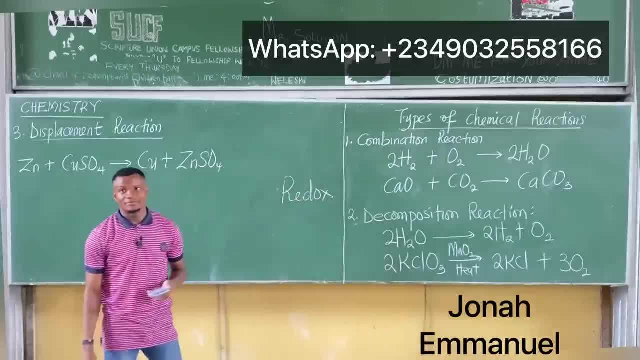 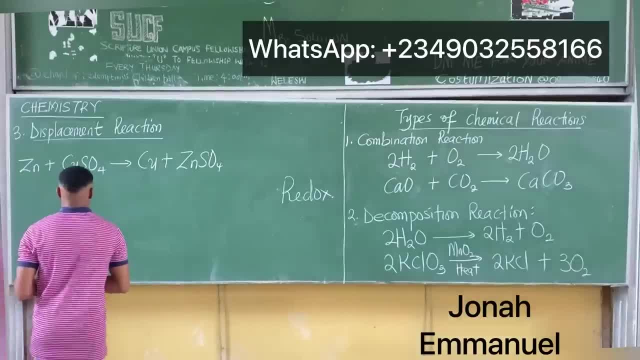 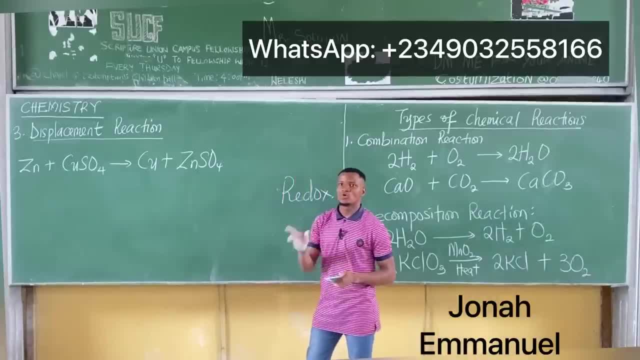 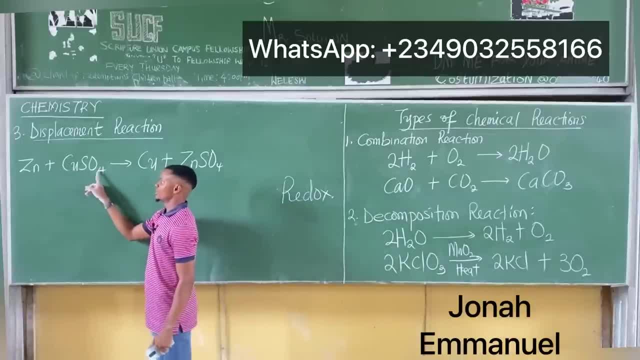 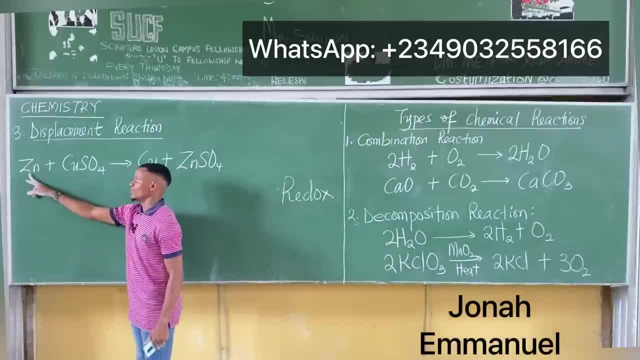 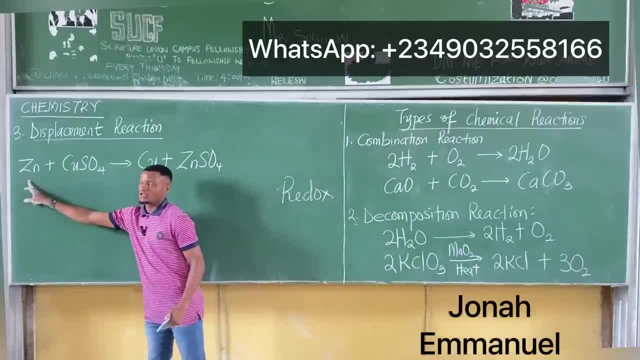 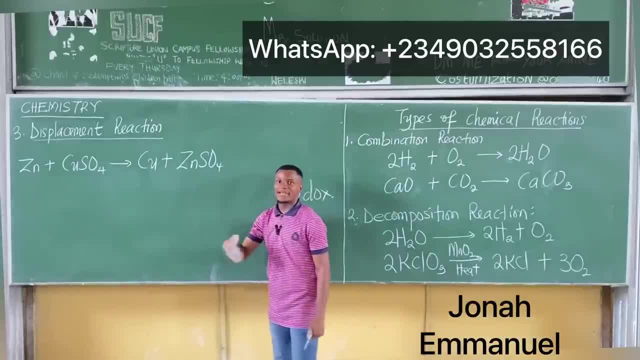 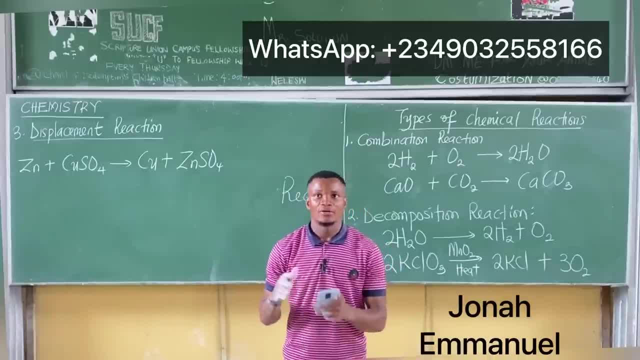 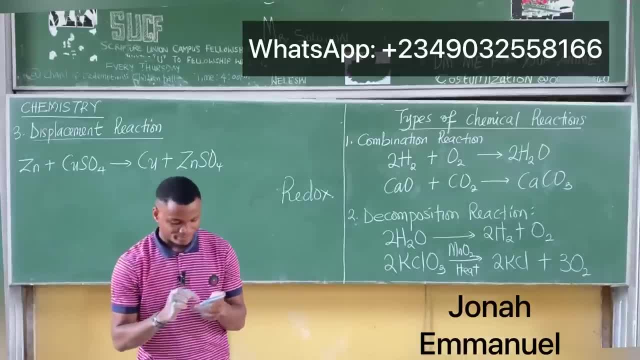 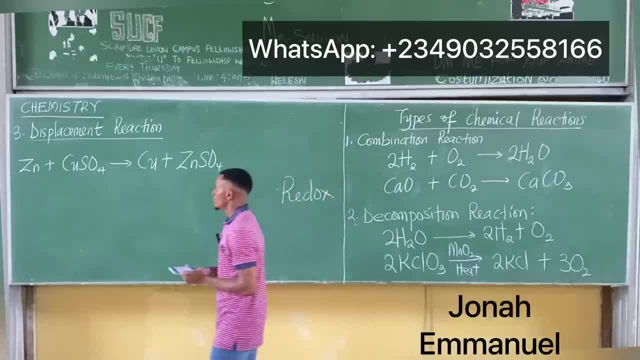 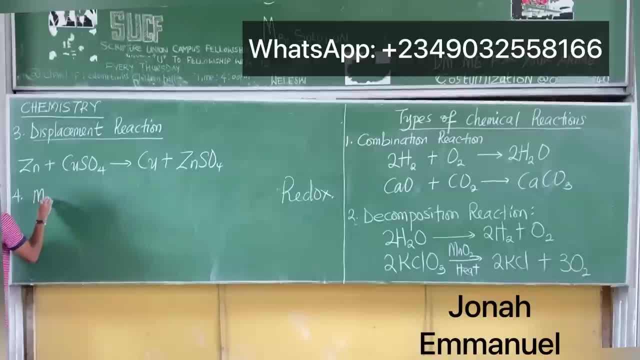 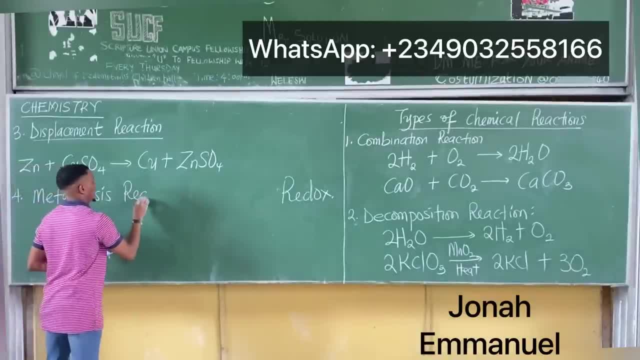 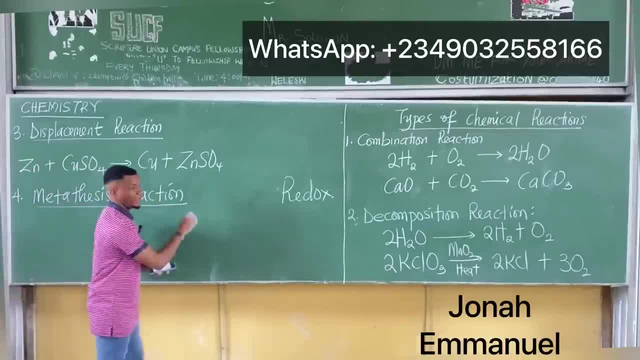 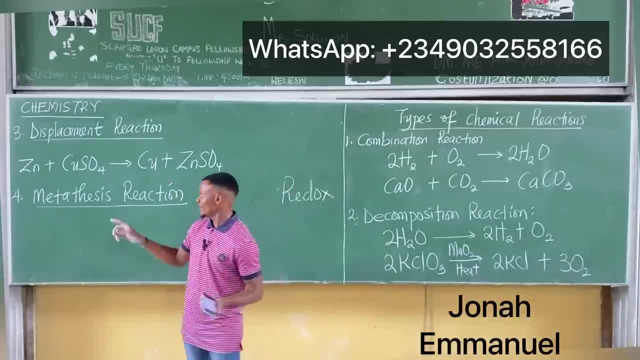 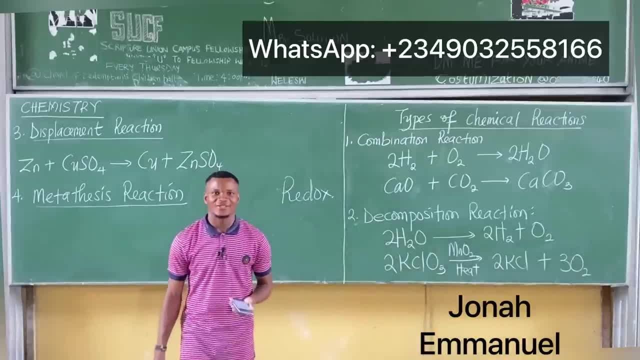 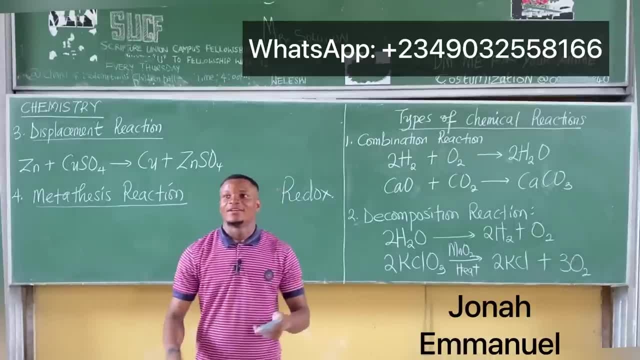 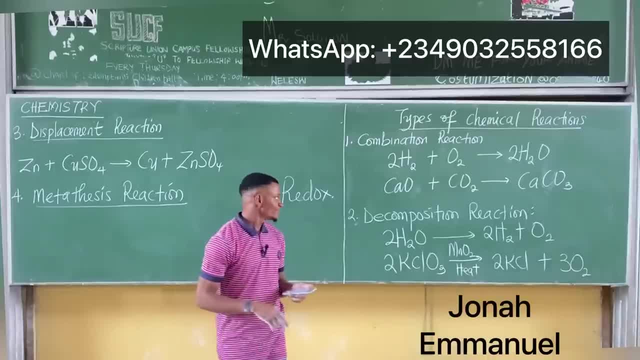 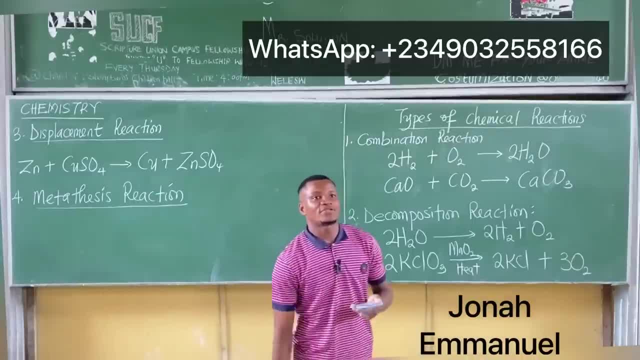 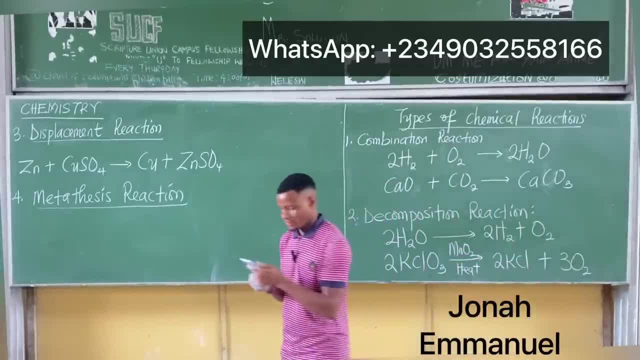 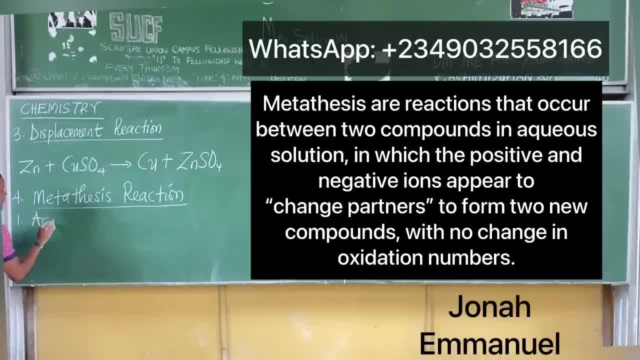 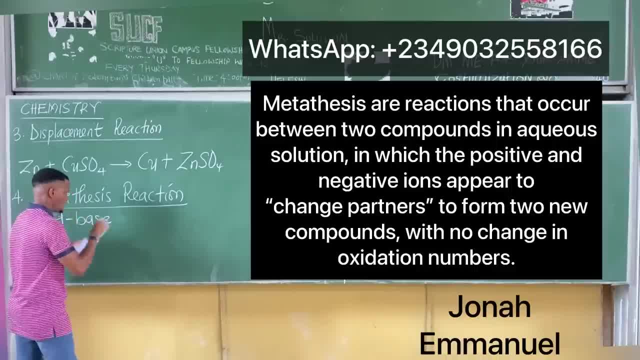 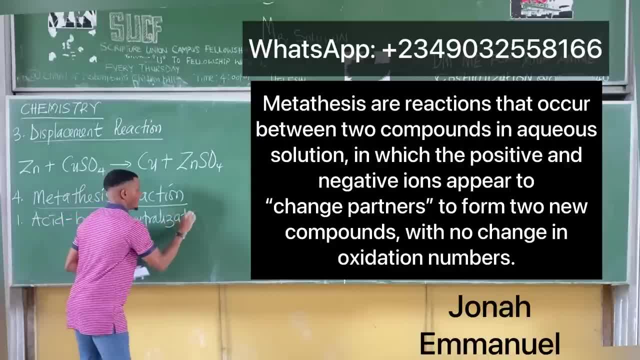 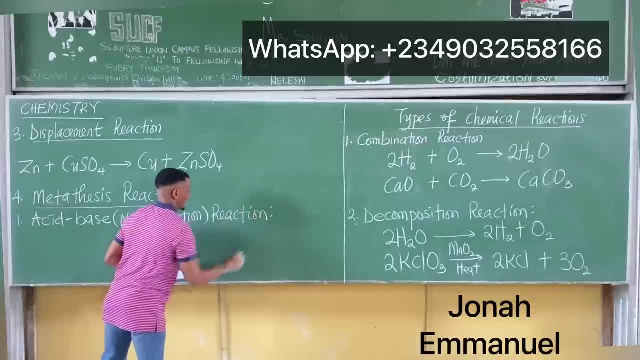 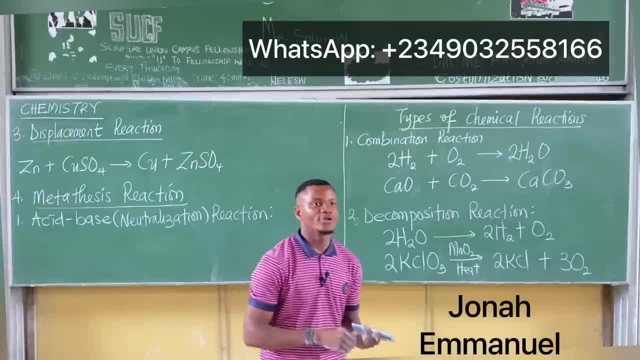 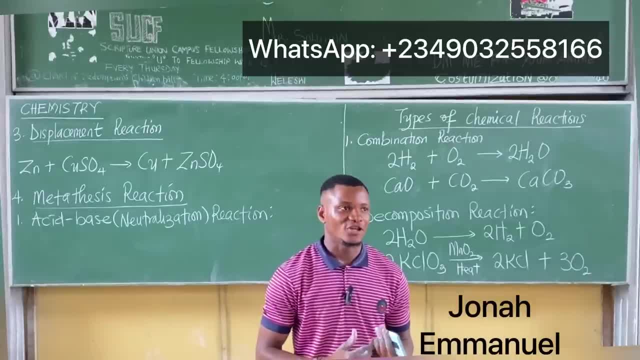 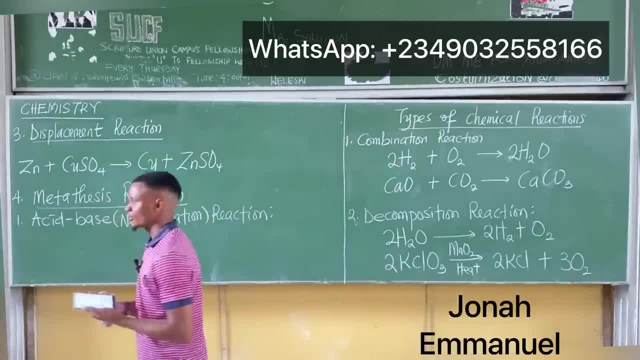 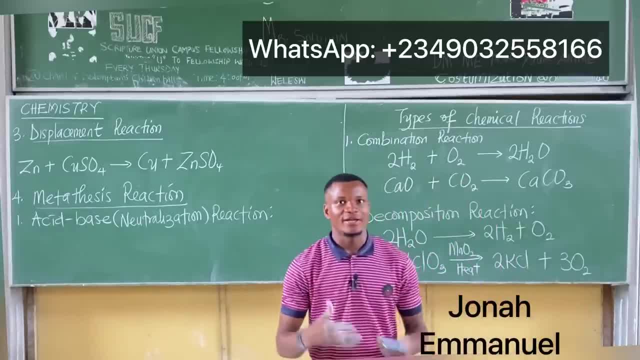 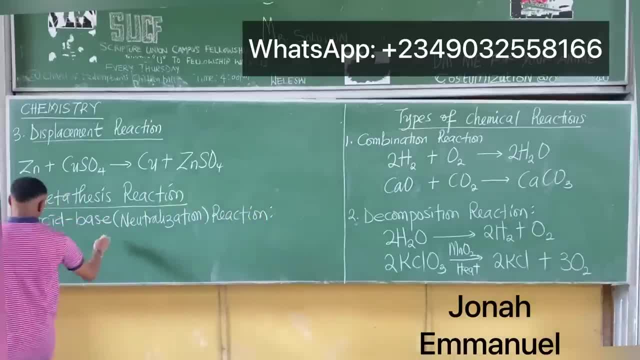 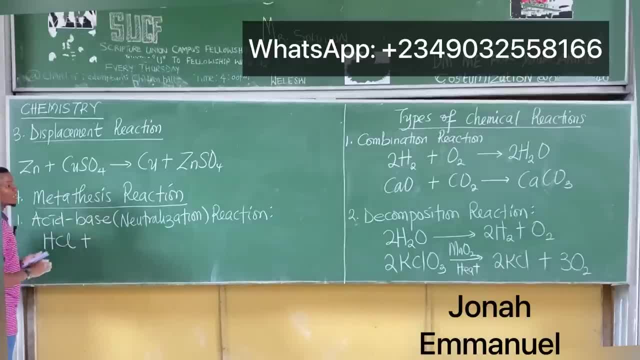 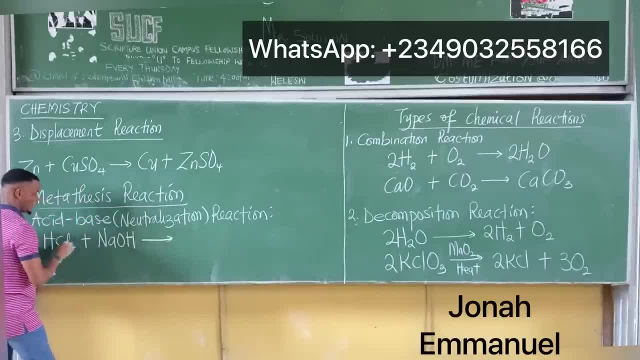 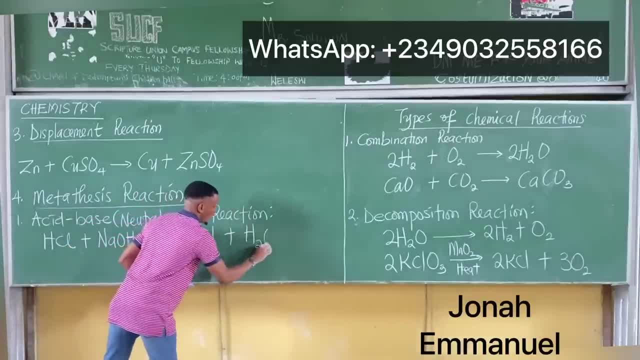 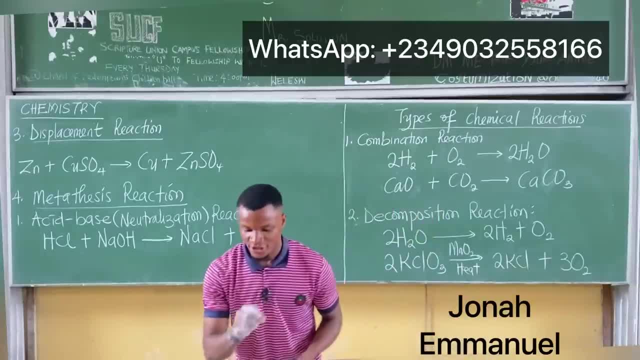 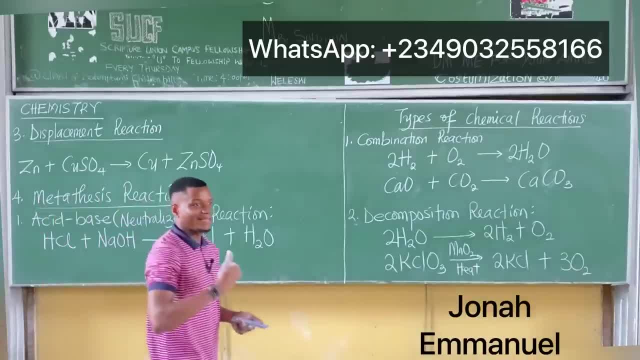 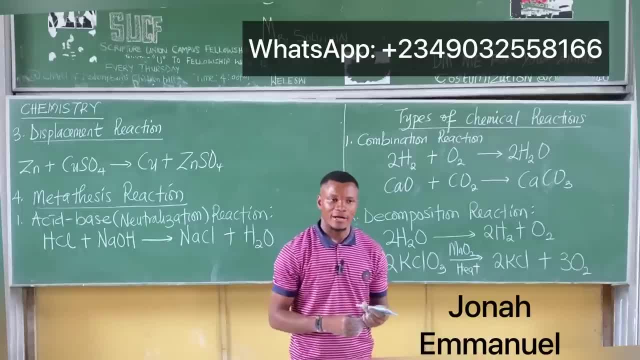 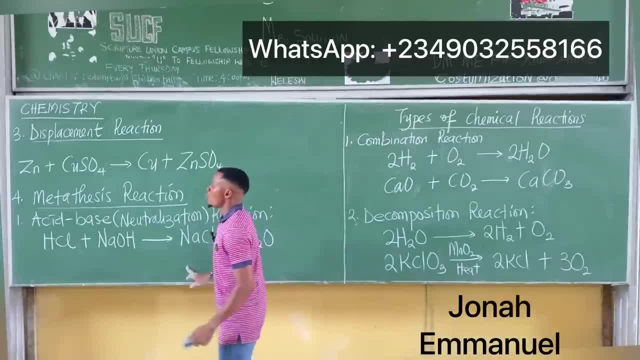 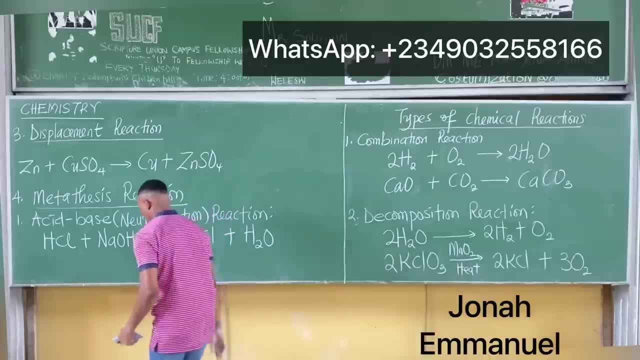 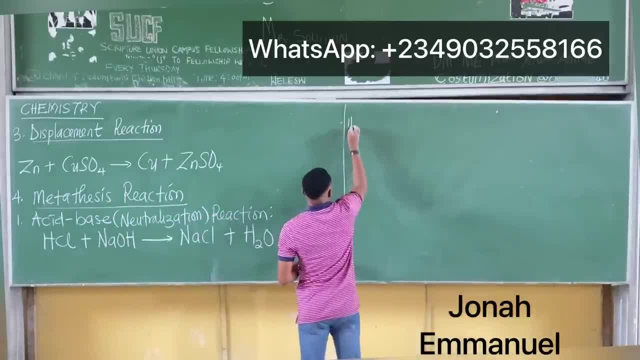 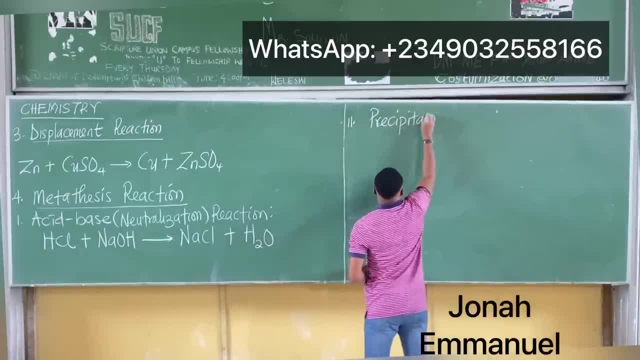 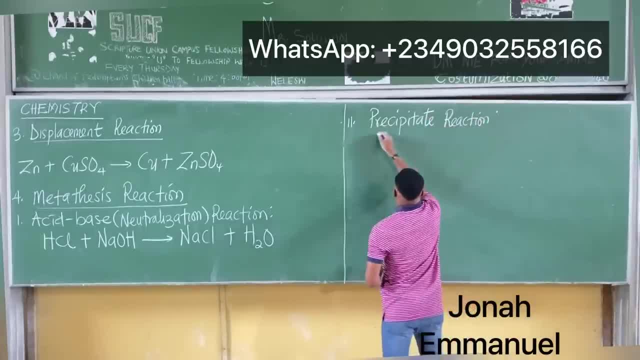 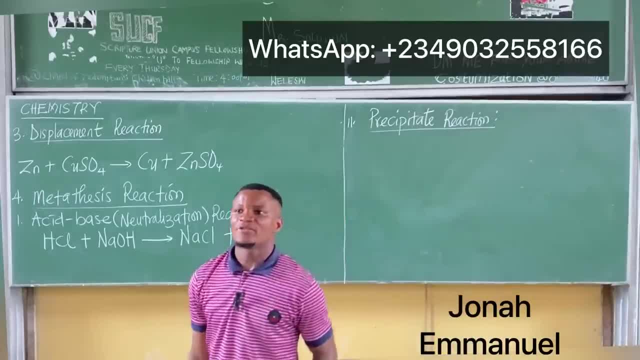 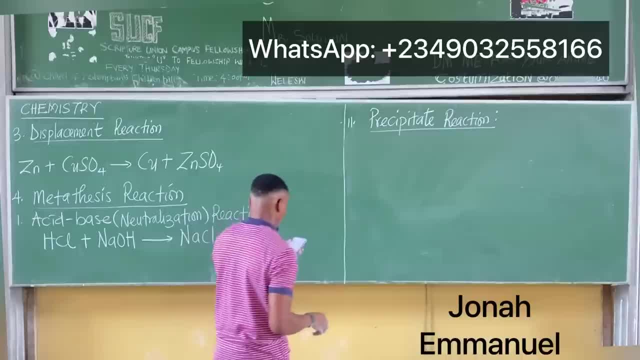 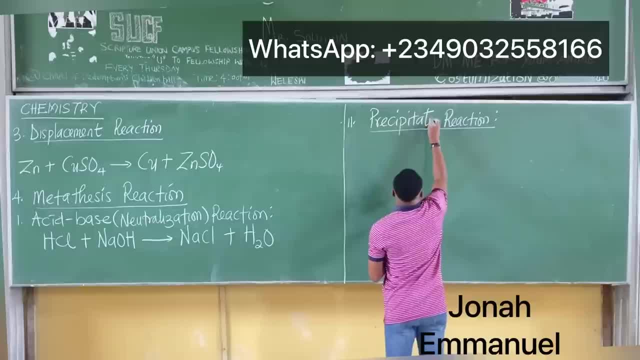 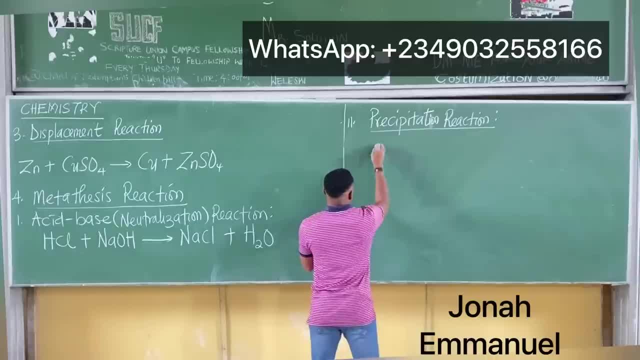 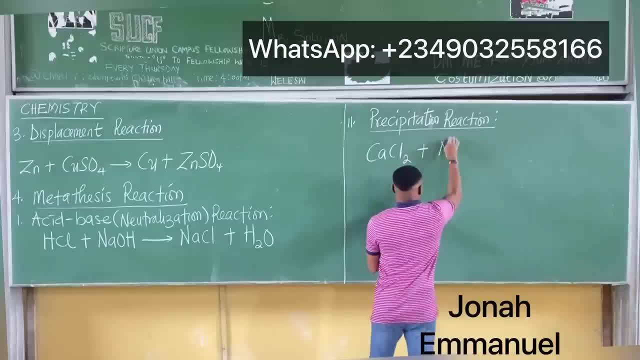 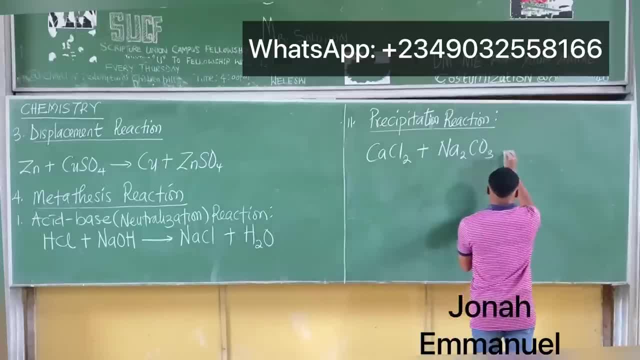 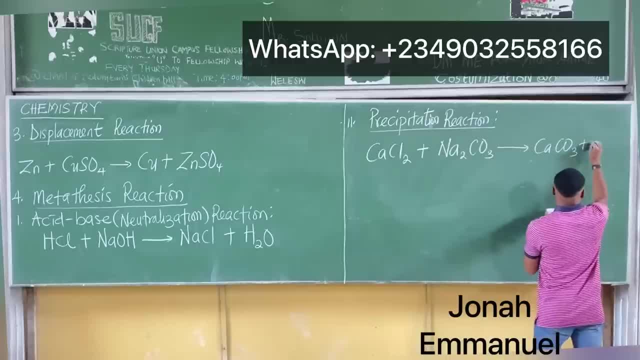 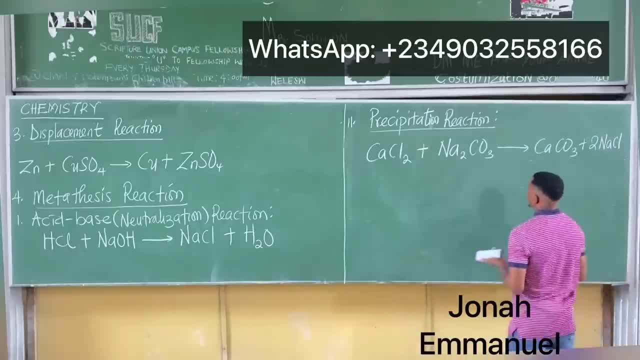 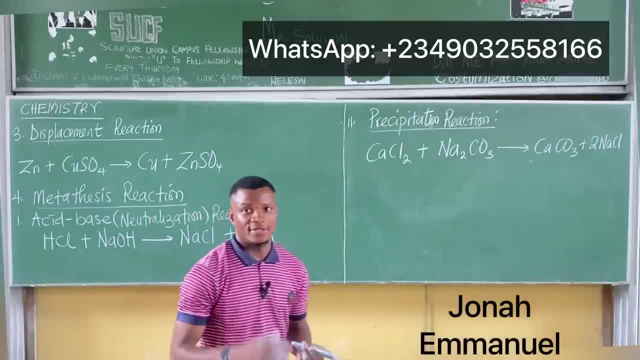 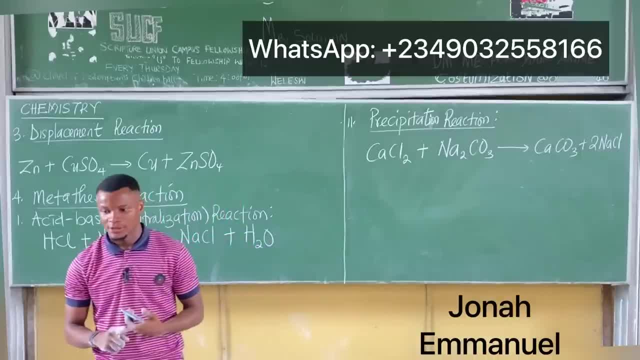 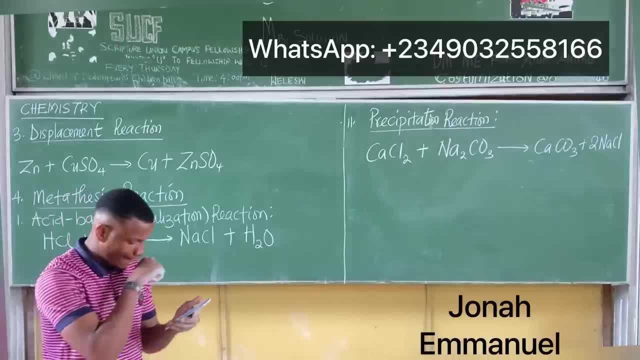 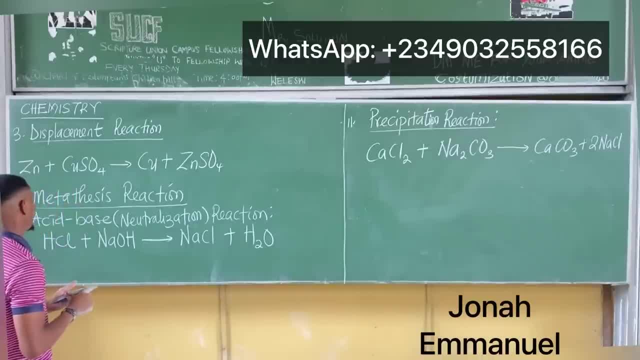 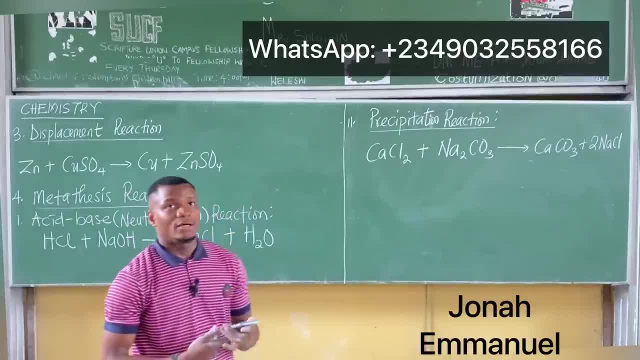 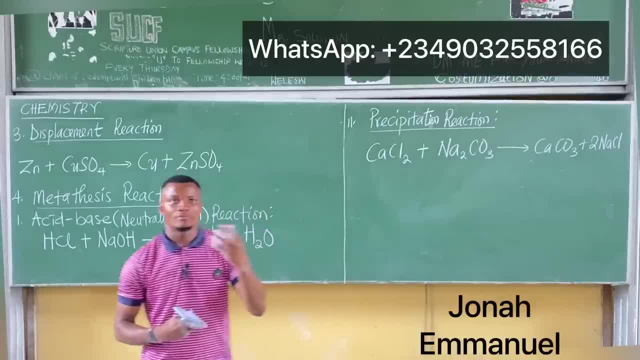 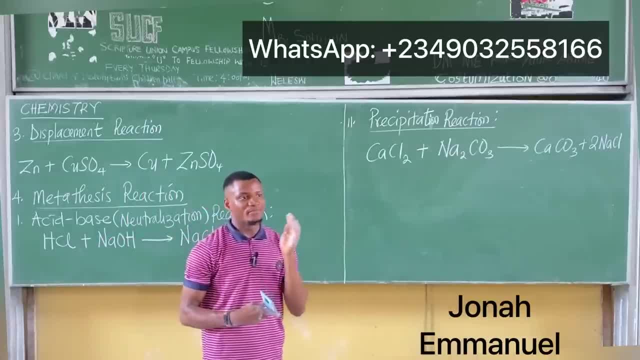 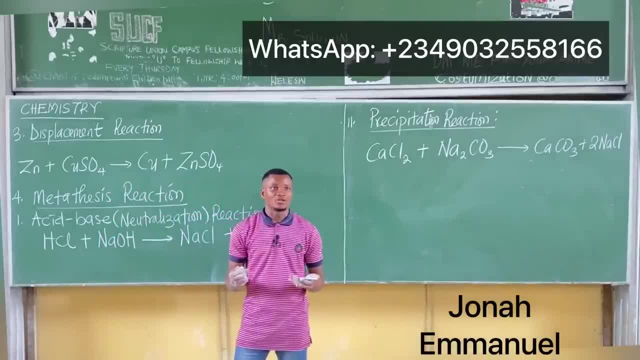 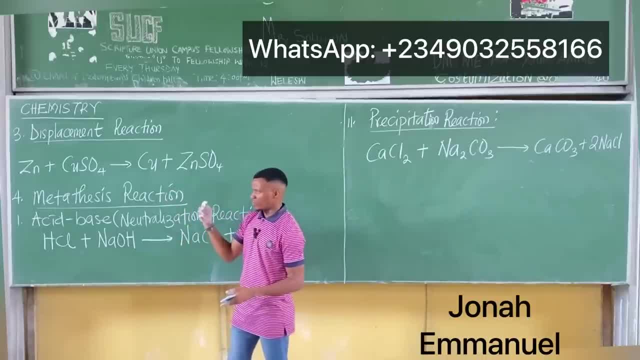 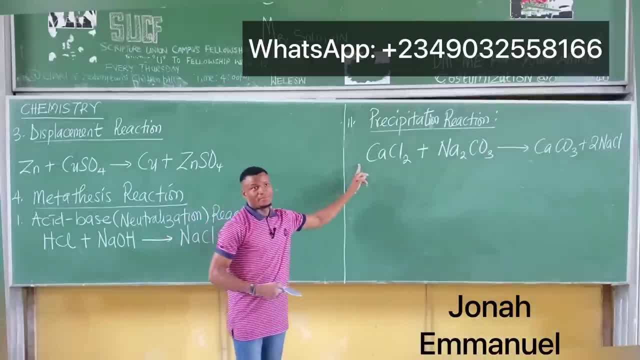 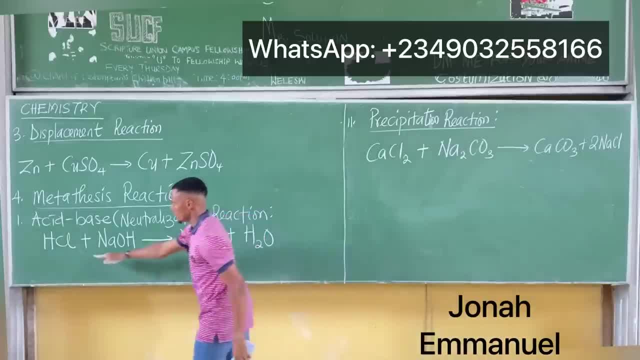 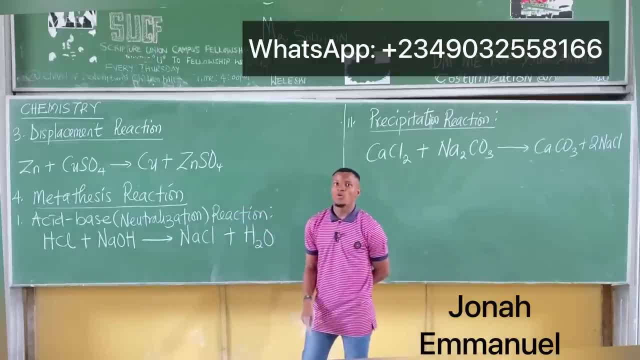 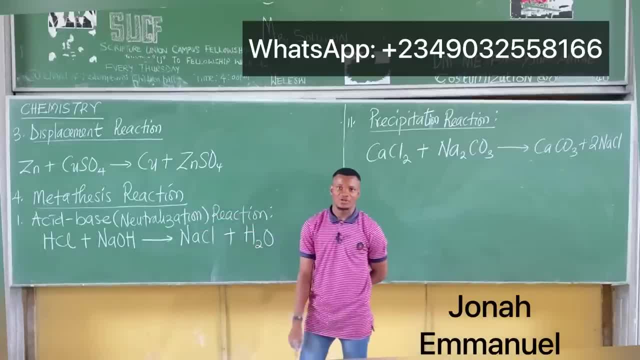 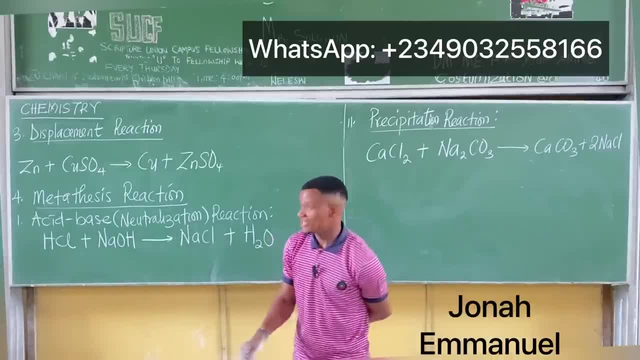 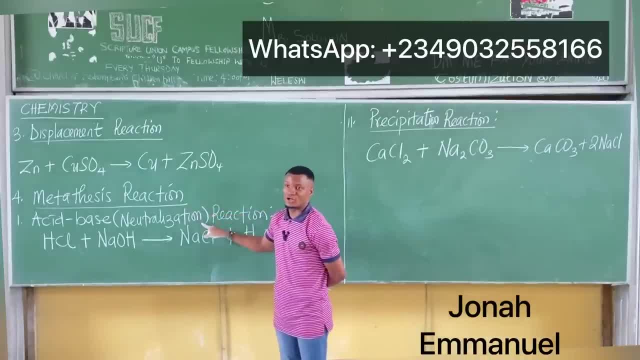 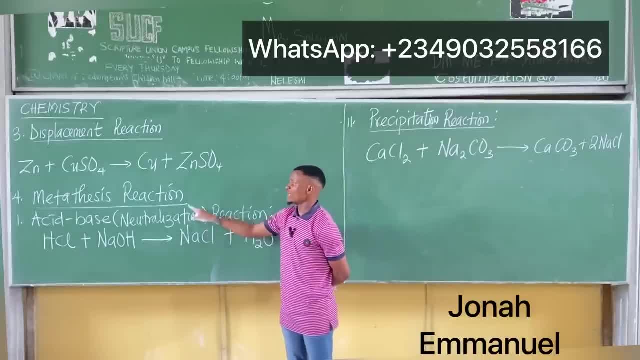 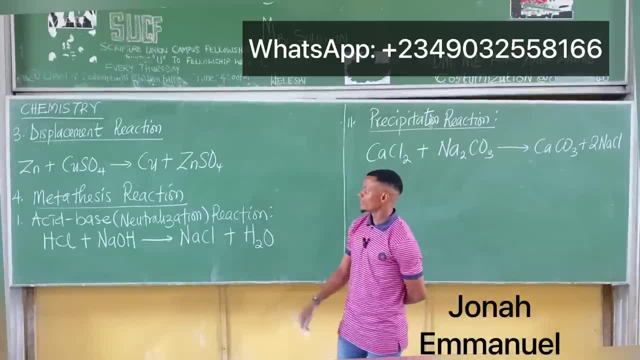 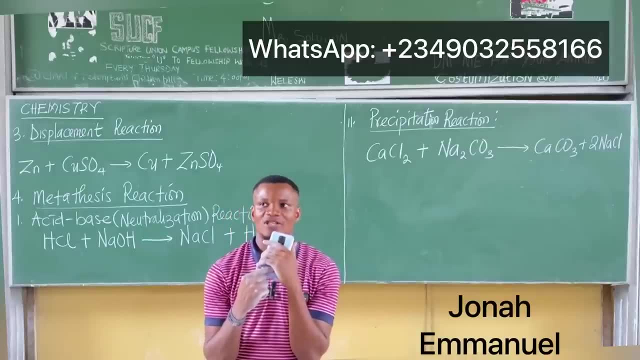 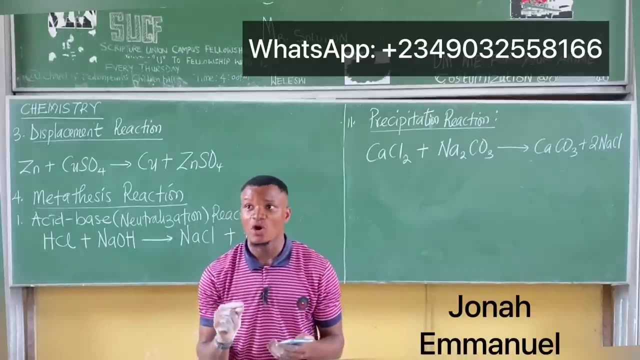 So please always pick out neutralization. How do you identify a precipitation reaction? That's the question, Because literally you have to actually do the reaction first and see the precipitate. There's always a hint, Listen, there's always a hint in the question. 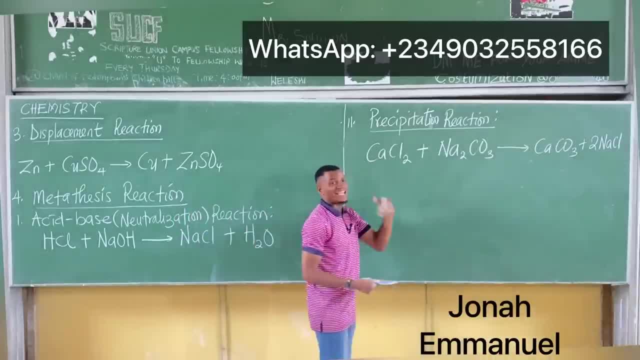 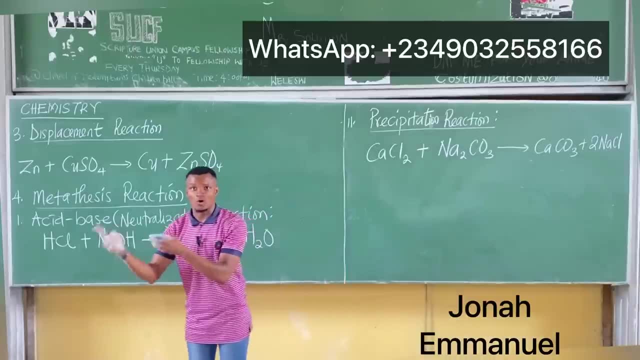 If you go to the past question, they don't expect that you should know all of this. They expect that you should know this one. Of course, if you're going with basic chemistry, you should know this: What is an acid and a base and a salt and a water? You should know. 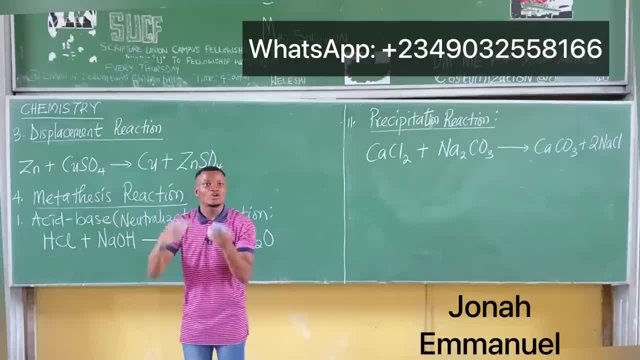 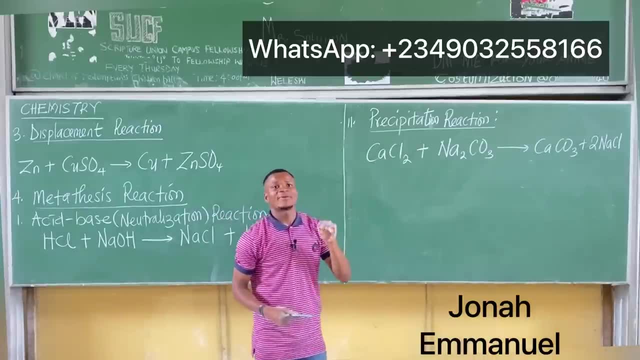 What is a combination? You will know Small, small, bigger one. What is a decomposition? You should know Bigger, small, small. But you cannot always tell precipitation. So how do you always remember precipitation? Read the equation carefully. It will give you a hint. You'll see equations like: 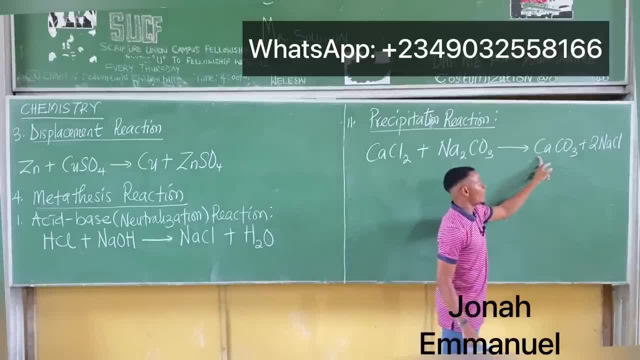 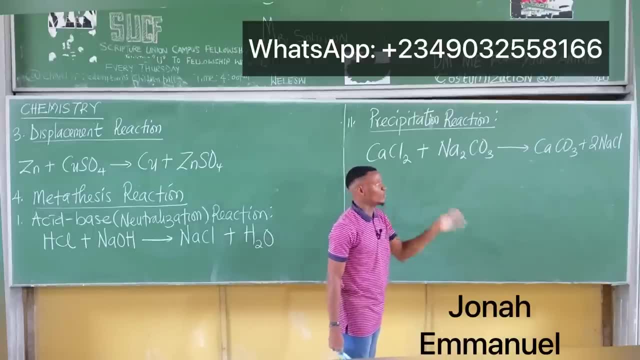 in the formation of calcium transcarbonate 4, using this and this comma, where a precipitate is formed according to the reaction below, And I'll give you this Now- I ask you: what kind of reaction is that? The answer is: 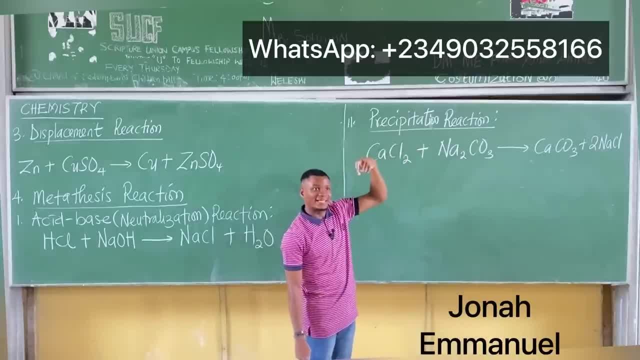 precipitation. The idea is this: They always give you that hint there That a white insoluble substance is formed. We'll give you that code there, So that tells you that it's what there- Precipitation. So always look out for that. 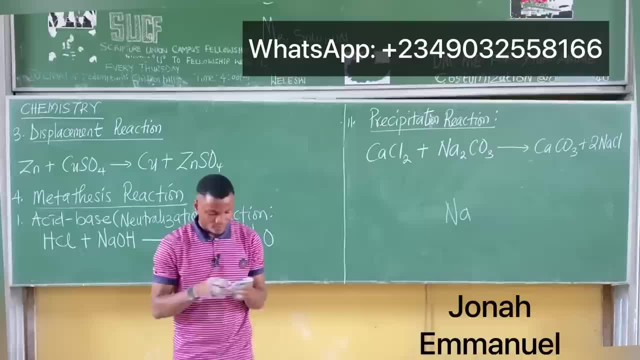 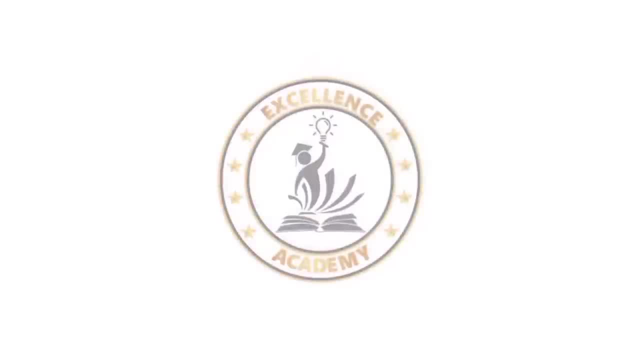 thing there. We'll give you that hint there And that's it Alright. I think at this juncture we can take a break. We'll be right back.